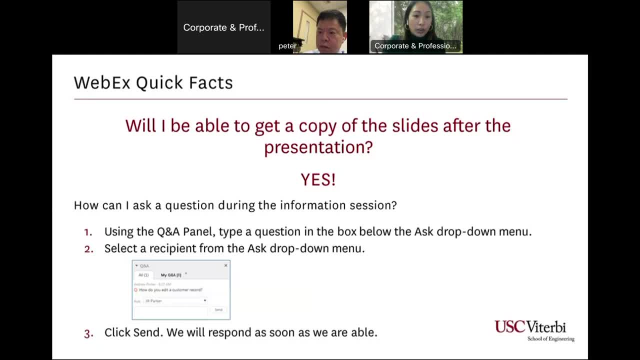 And so then we'll be able to monitor and be able to answer those questions. you know especially, you know, towards the end we will be having a Q&A session where you can definitely ask your questions to Professor Wang and he'll be able to answer those for us. 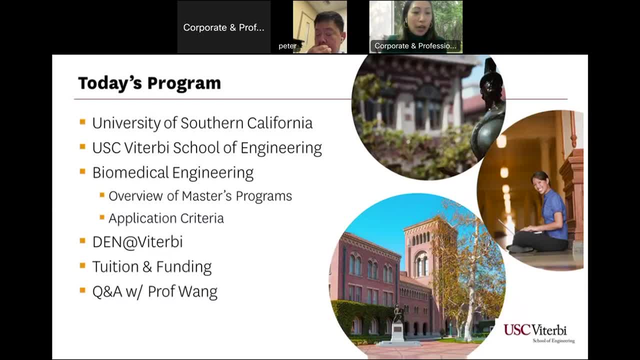 So, for today's program, I will give a quick introduction of University of Southern California, Followed by, you know, just some information about our own Viterbi School of Engineering, And then I will go ahead and pass the presentation over to Professor Wang, who will then, you know, talk about the different file management engineering programs and give you an overview of the master's programs themselves. 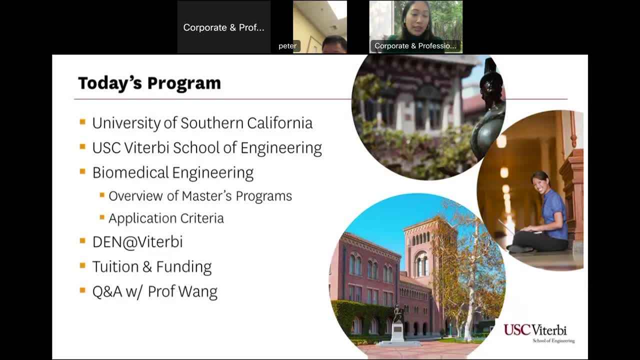 And then about the application criteria. I'll then continue and you know, go through our DNF Viterbi, which is our online service, And then talk a little bit about tuition and funding, and then we'll end this webinar with the Q&A session with Professor Wang. 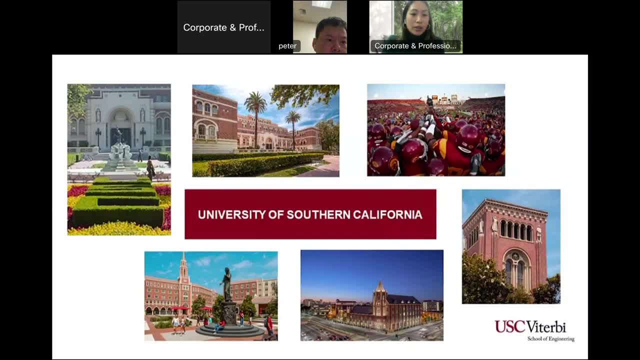 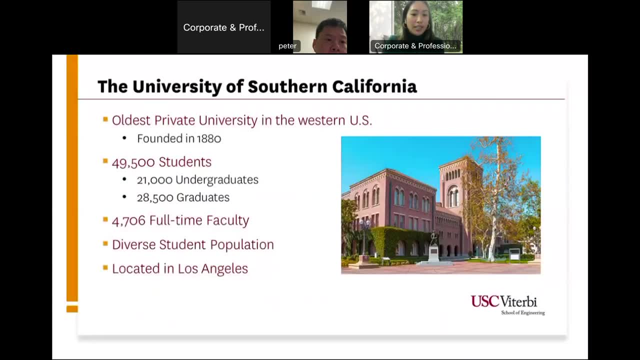 So here's just, you know, some, some photos of you know of the campus which is located in Los Angeles, And you know we are the oldest private university in the west of the United States. You know we were founded back in 1880.. 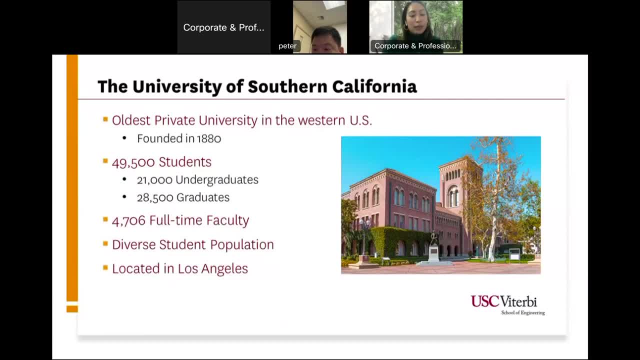 And also in 2018.. So we are the oldest private university in the west of the United States. So, in terms of the student population, you know we are, you know, almost close to 50,000, in which you know our graduates are, we have more graduates than our undergrads. 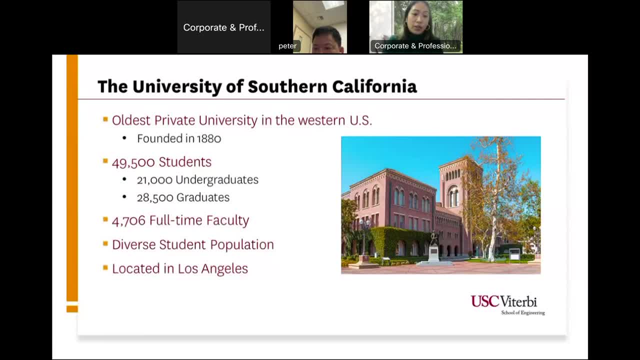 And then we do have, you know, over 4,700 full-time faculty across. you know, the entire University of Southern California, And these are also including our adjunct faculty members as well. you know who you know come from. you know the work industry. 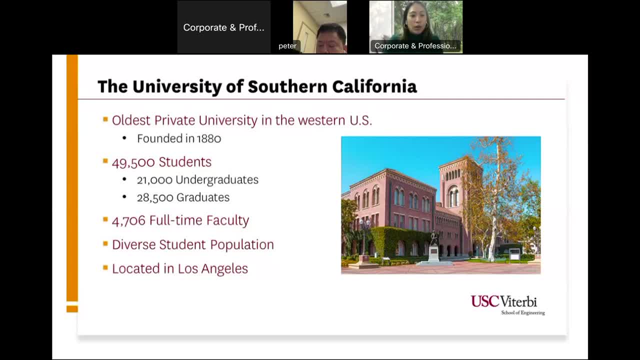 And they're able to bring you know information and expertise from the workforce you know into the classrooms for our students. We do have a really diverse student population. Our students come from all different walks of life, from different industry backgrounds, as well, as, you know, just all over the globe also. 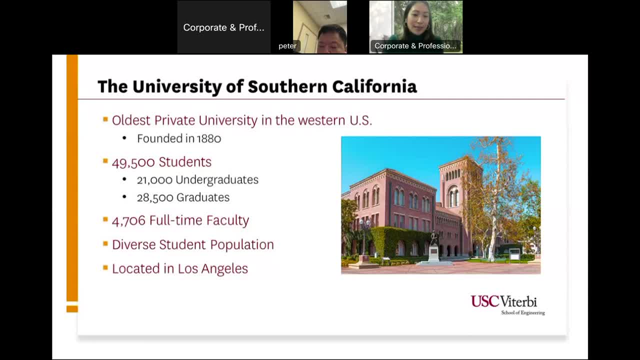 And, as mentioned, we are located in Los Angeles. So just a quick summary. So we are located in Los Angeles. So just a quick summary. We are located in Los Angeles. So just a quick glance at Viterbi School. 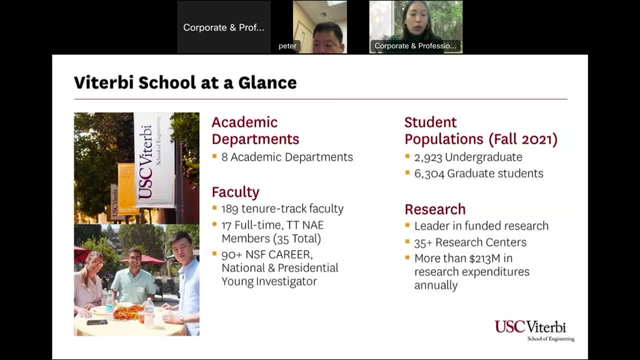 We are made up of eight academic departments, where biomedical engineering is one of the eight, And then we do have 189 tenure-track faculty and 17 full-time, 33 TTNAE members as well, And then over 90, actually National Science Foundation, career national and presidential young investigators. 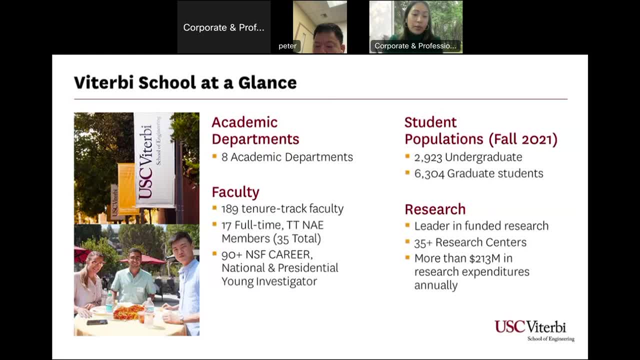 And I'm going to jump back into our faculty. You know Viterbi School is the leader in funded research. A lot of our faculty, you know, spend their time alongside with our doctoral students in conducting research in more than 35 research centers that we do have. 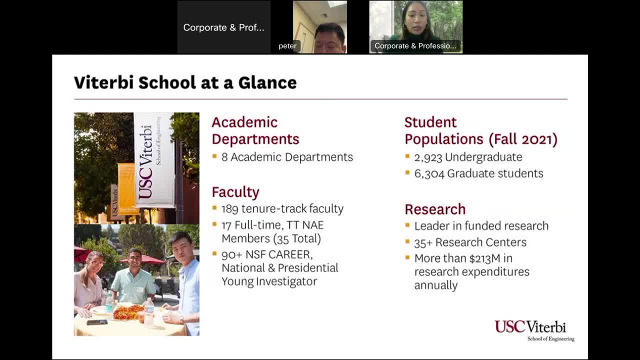 And also there's more than $213 million which is invested in research expenditures annually In terms of student population. you know it is—you know it's very small and it's very small and it's a little bit closer to the cost of the program. 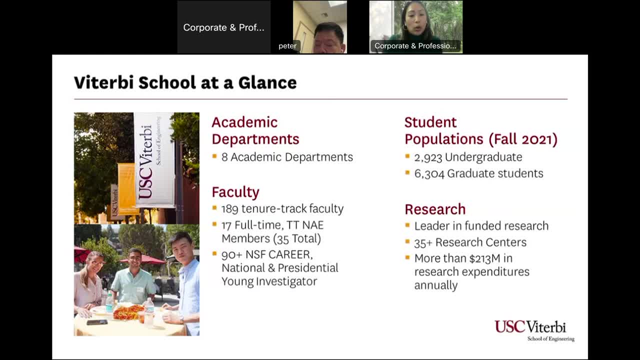 And so you know, we begin with the most recent student population. You know, it is actually, as you can see from this slide, that our graduate students is almost tripled the amount of our undergraduate population, And that does include of our master students, our graduate certificate students and our PhD doctoral students. 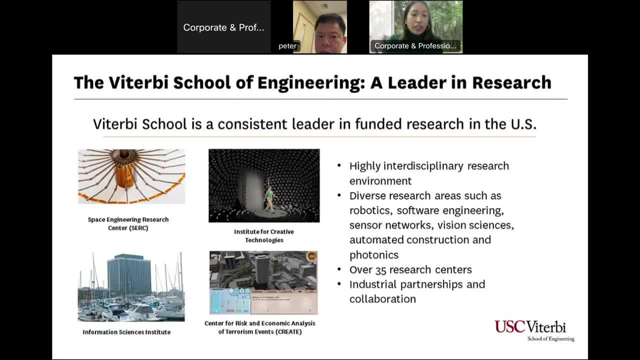 And just really quickly tying into research and, as I mentioned, the school is the leader funded research We are. you know it's a very highly interdisciplinary research environment. We do have over 35 research centers. We do encourage you to visit our website If you are interested in learning more about our research centers, to to just kind of see what the different research offerings are available. 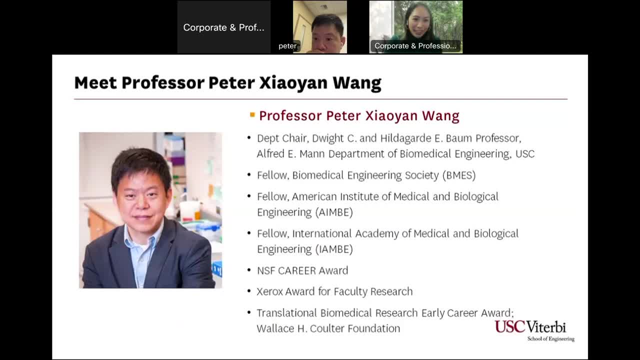 So, for today's purpose- you know we're going to be talking about. You know we are here to to meet with Professor Peter. So, Professor weighing, you know, as you can see from the slide, you know he has received so many awards. you know has a fellow as well. 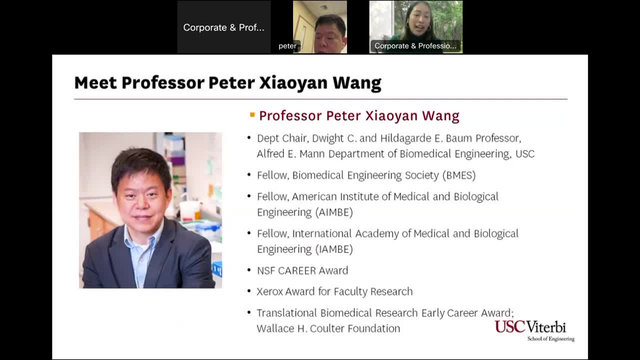 And he's just very, very, very experienced. So you know, we're very, very happy to welcome him, you know, and he is, you know, the current department chair of our biomedical engineering program. So a very, very warm welcome, Professor weighing, and I will go ahead and let you 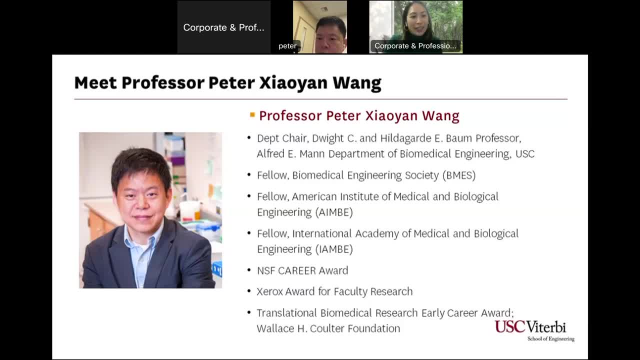 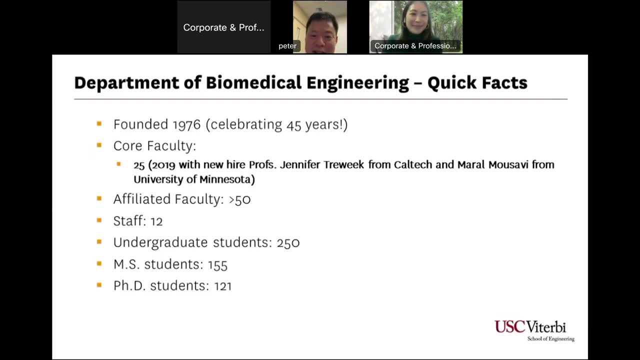 Take. take this forward and I'll go ahead and navigate the slides for you. Thank you very much, Mary. it's also a great pleasure seeing everyone. So I just started the you know, my new position here at USC. Actually, Mary, can I see myself? somehow I cannot see myself. 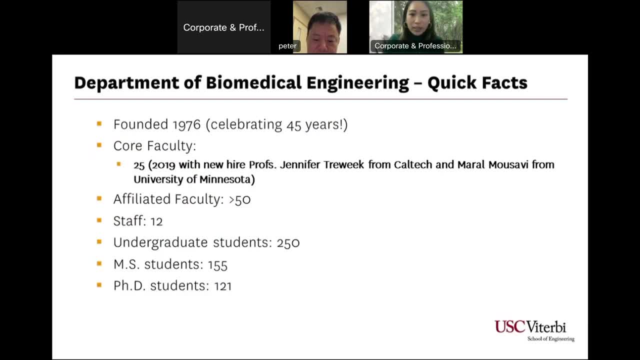 Is there any way you can? Yeah, I could. Yeah, Let me see. Okay, Can you see yourself now? No, I don't know whether it's my setting or Yeah, it's fine, You know, I can just keep going. 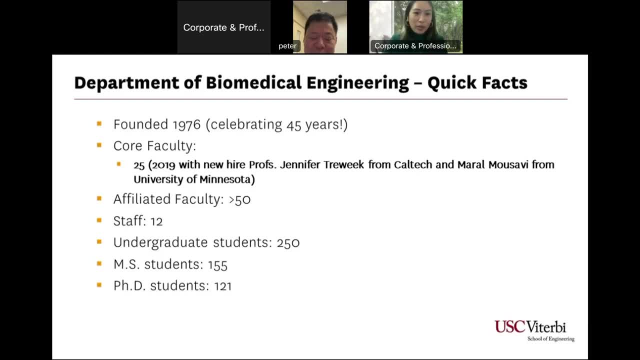 Okay, Yes, we could see you, We could see you. Okay, We could see you perfectly. Yeah, Okay, no problem, Yeah, so basically, you know I'm somewhat new, you know already had a lot of time. 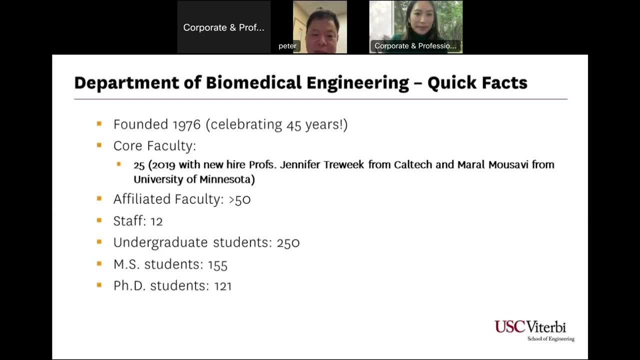 a good time together with colleagues and students here. So I was a professor at UC San Diego in bioengineering, Stayed there for 10 years and just recently moved to USC. Now I'm like three months into my new position. So for my department, as you can see from the information list on the slide, 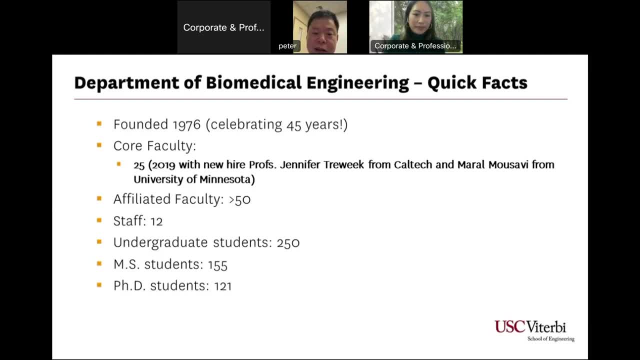 we have a really really long history right. It started in 1976. So one of the most established program- I think we are probably the first at the West Coast- And we also have 25 or so core faculty covering a broad range of different areas. 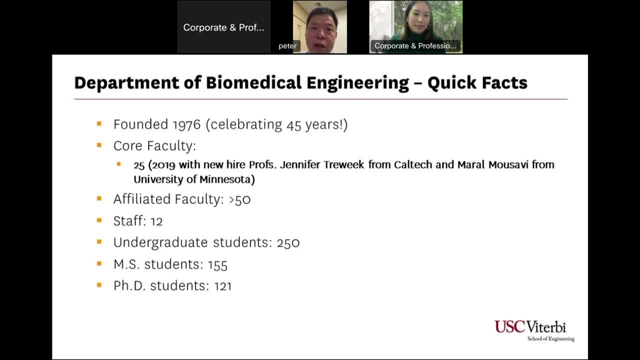 Biomedical engineering from like modeling, analysis, imaging, drug delivery, medical device, as well as neuroengineering and the cellular and molecular engineering. Essentially, we try to engineer the cells and genes and also, using, you know, equipment, the device to control those genes. 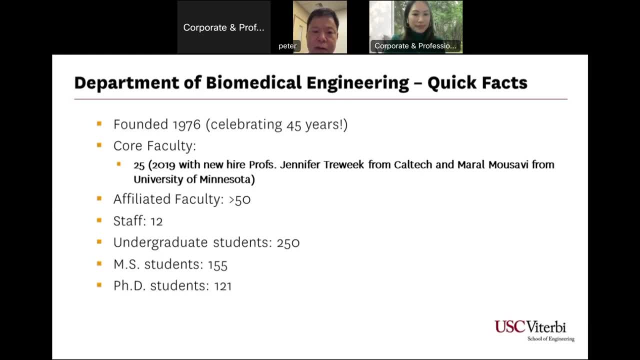 and the cells, And we also have a larger pool of affiliate faculty, So essentially students can have no problem finding any. you know specific area you are interested. We have like more than 50 affiliate faculty across different units and academic departments at USC, Many of them actually. 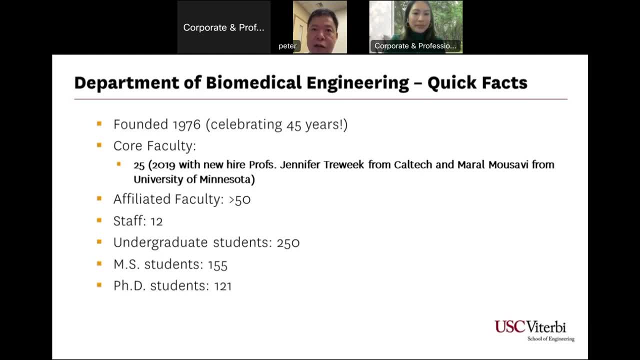 are from Keck School of Medicine, So if you are very interested at the interface between engineering and medicine, particularly applying the cutting edge technology in engineering approach to medical applications, you will find the opportunity to work with them. You know, in any direction it's a top-notch talent to work with. 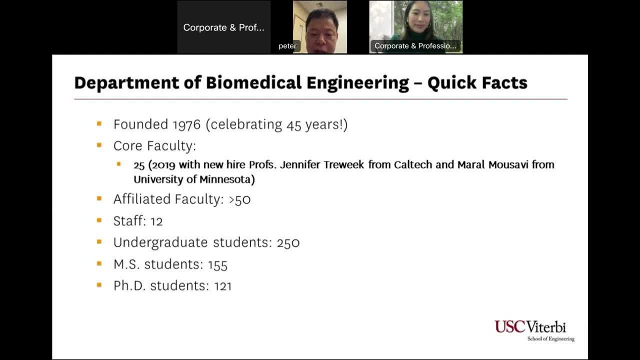 Currently we have 155 master's students and 121 PhD students. you know across the years, So you will find out. there's a very enriched environment. You have a lot of chance to talk to students and learn more about the- you know- evolving field of biomedical engineering. 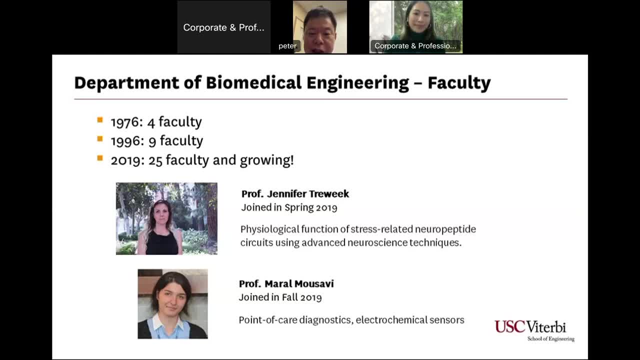 Maybe next slide? Yeah, so we are continuously recruiting. you know the new talents and new faculty, As you can see here, when we started we only have four like funding. you know faculty right, And then you know there's like a growth very, very slow. in 20 years We only have, like you know. 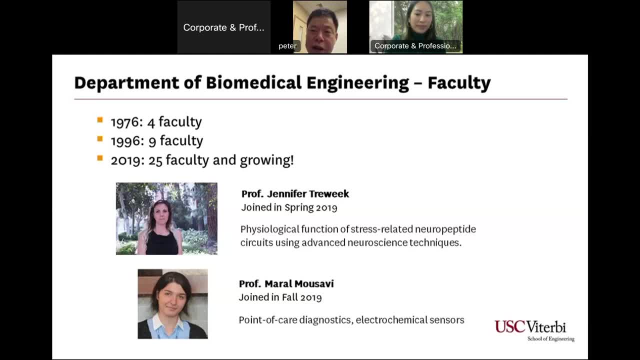 nine faculty And then you know there's a relatively fast growth And now we have, more than you know, 25 faculty. Professor Jennifer Truik was, you know, recently recruited from Caltech. She's basically an expert. 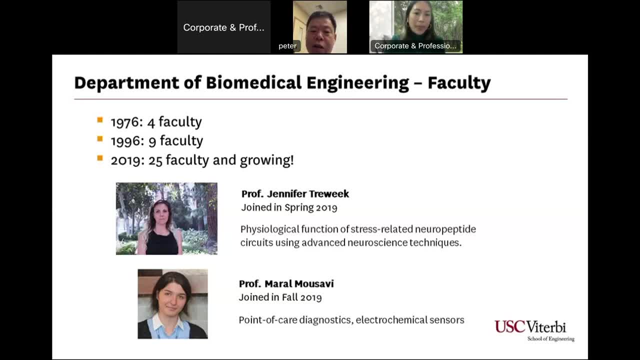 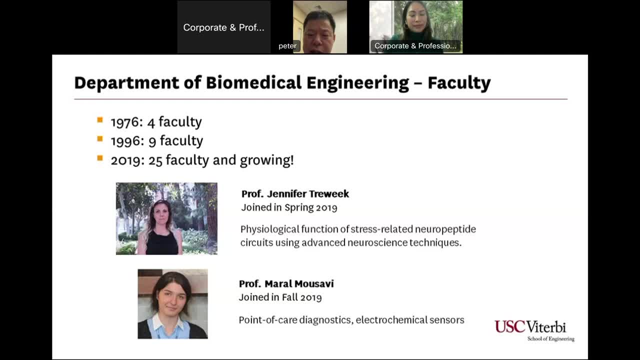 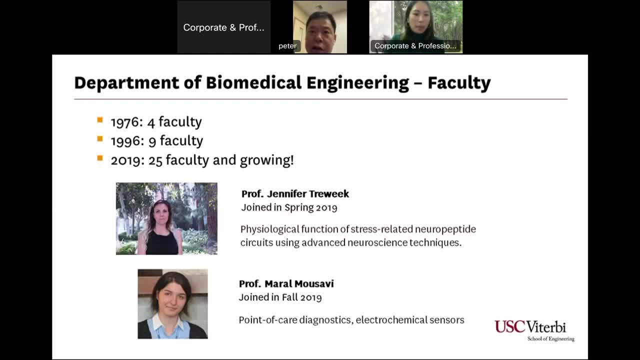 And this year we also have, you know, a position. hopefully it will be more. So basically, we have 350 faculty applying for our position And we're now down to seven. you know really top-notch faculty and we are really actively trying to recruit them, Hopefully. 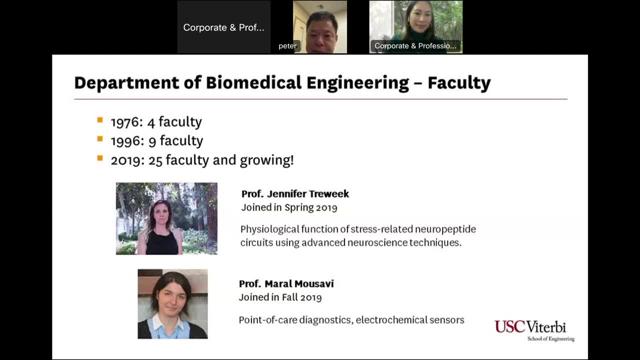 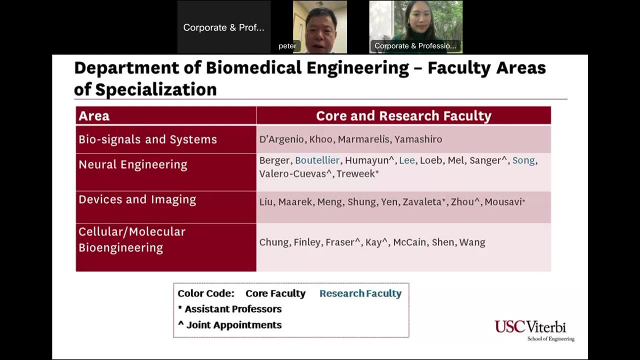 we can at least have two or three you know faculty joining us. Okay, So these are the like general information For the department. you can already see from the you know charts. we have multiple areas focusing in the department at the current stage, covering, for example, 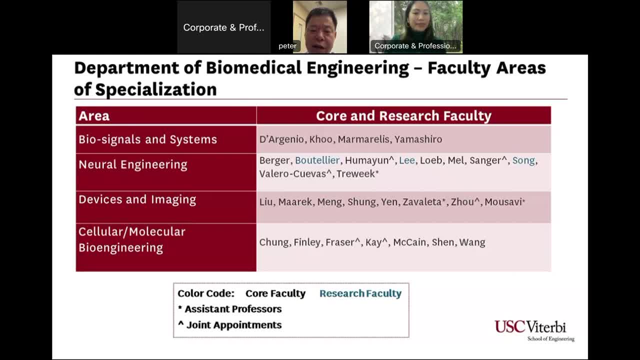 power signals and systems. We have a professor Di Eugenio, Marko Khoo, Vassilis and also Yamashito, So these are basically the early kind of roots when we developed the department And now we also grow in the Neuroengineering area. 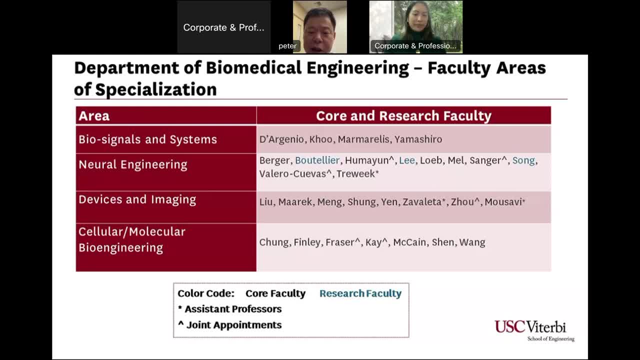 We have Ted-Berger, you know, Homaya and I don't want to list, you know each engineering video faculty here, but it's actually strong and big group. we have like one, two, you know totally. we have like nine or ten people you know in this area. we also have a very, you know, strong. 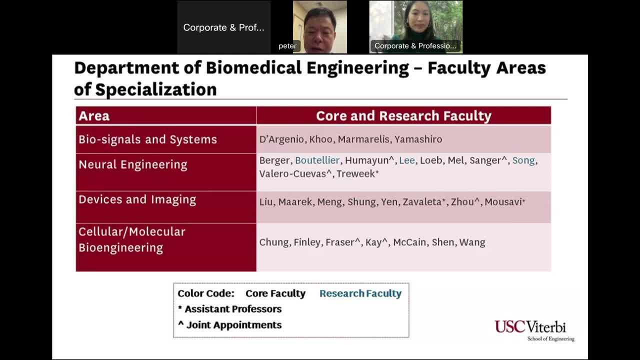 device and imaging group: uh, right now we have totally like uh eight faculty in this area. sorry, because i'm using my cell phone so you know some of the words are kind of small for me to read. again, this is also strong, you know, group in the department. now the last group was cellular and 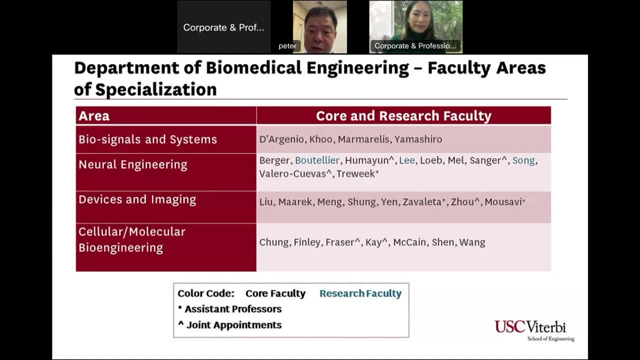 molecular bioengineering, although it's somewhat relatively small at the moment, but it's a rapidly growing thing. you know. you already see quite some. you know, like active faculty in this group- and myself also should belong to this group- and we are continuous continuing, you know, recruiting people in this area. uh, next, please, yes, thank you. so in terms of the master program we have, 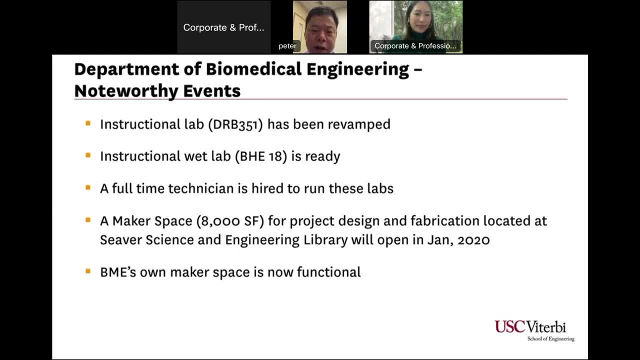 several. you know, uh, like a different. uh, you know directions and, uh, these are the. you know development across these. you know years. uh, we already have instruction instructional lab- uh, you know, basically renovated and also the wet lab space is also ready so students can have hands-on experience. if you know, some of you are interested to play with the real, like cells, genes. 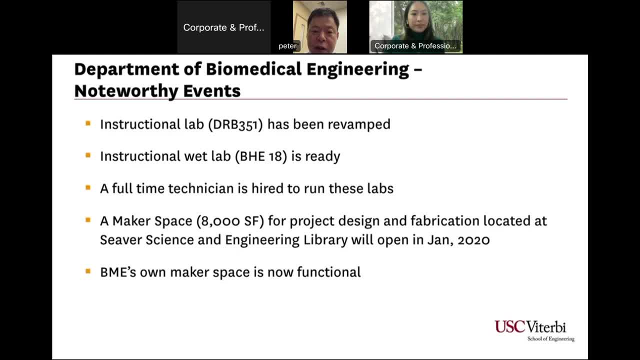 and device you know. so you have a place to play with uh. and also we recruited a full-time technician to help to run those labs. so students can not only learn the contacts, the principles in the class and lectures can also really- you know, play and have fun. we also have a make space area: 8 000 square feet. 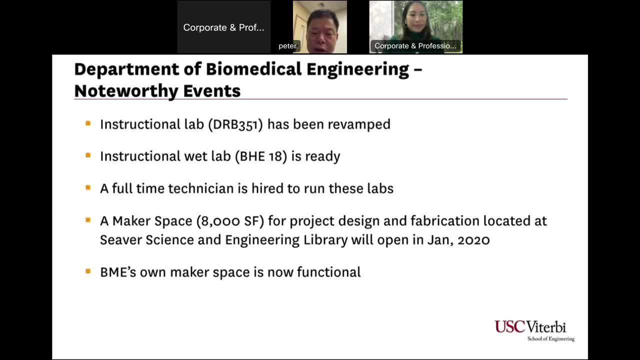 for the project design and fabrication, which is, uh, you know, located at the silver science engineering library. so, again, that's a huge asset for us as well, for the student to have a lot of, you know, real hands-on experience. we also are creating this own maker space and now it's a 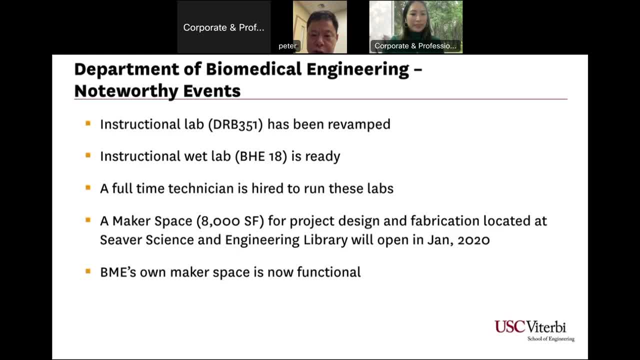 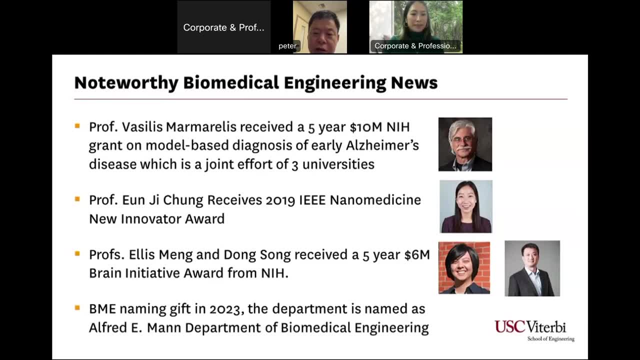 functional. so there's multiple options for you to choose to have your hands. you know our experience. next slide, please. so these are some, you know, recent development again, you know our faculties are continuously, you know, strive uh, you know really uh ahead in the different areas of biomedical engineering, particularly professor vassilis memorialis recently received. 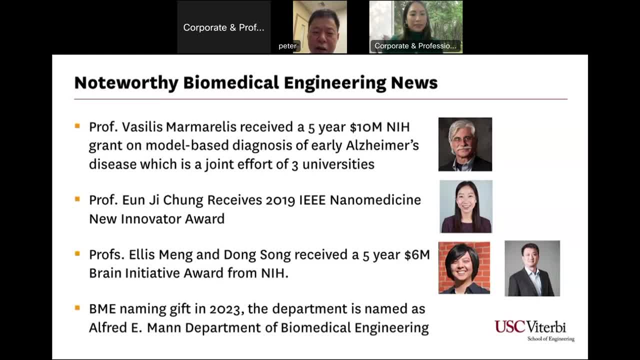 like 10 million dollars or a natural funding on model-based diagnosis or early as hummus disease, which is really a joint effort to multiple universities and uh professor onji chang, who received the, you know, the ieee nanomedicine new innovator award. she also was a winner or? 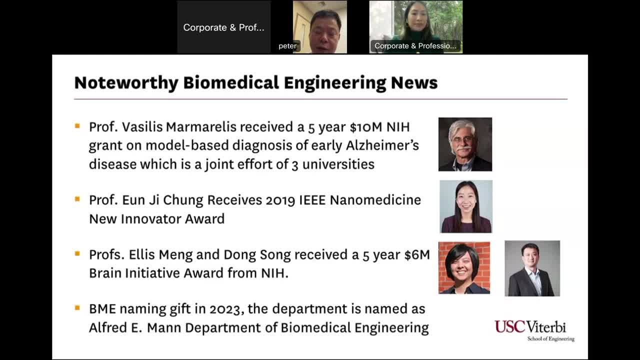 a nih innovator award, which is a big, you know, or grand prize for any young faculty you know. there's only, i think, several dozens each year from the whole nation. uh, our recent uh, professor maro masavi, also won the nh innovator award, just you know, last year, and professor alice. 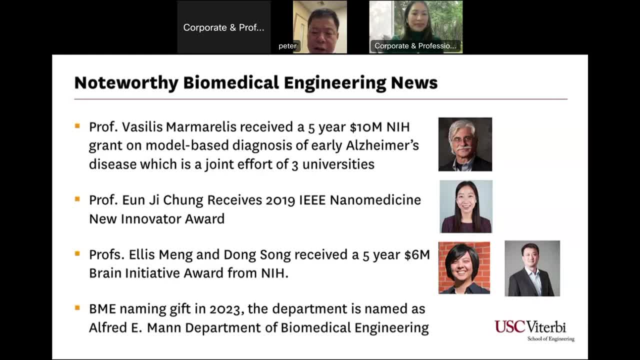 mann and uh tung song received five years six million brain initiative award from nih. they actually recently also had a major, you know, center grant. i think it's 11.4 million from nih. so again you can see that the integration between the device and the brain or neural engineering, 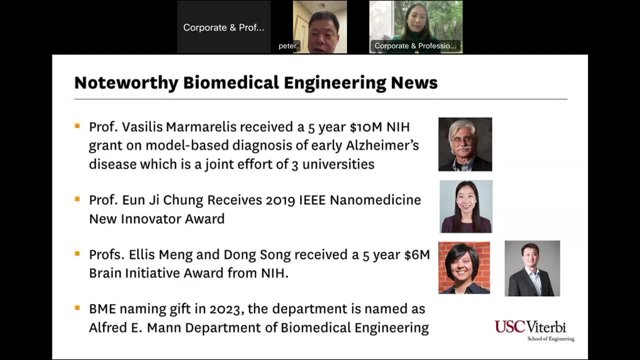 group, uh, you know, like converging and we are creating more and more active, you know, centers around those directions. uh, most recently, we are very fortunate, uh, due to, you know, the generous gift from alfred guinness, who is a professor at the university of california, who is a professor. 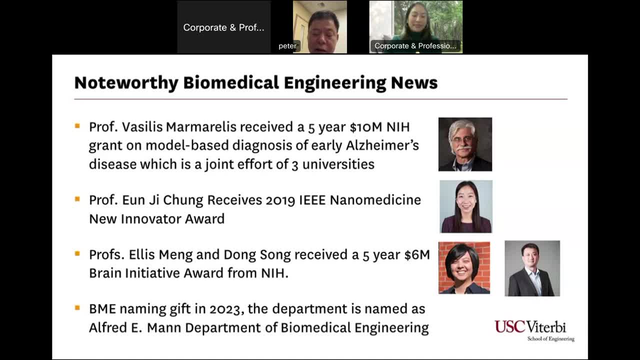 e main foundation. we really have endowed- or, you know, named our department as alfred e main department of biomedical engineering, and this gift is 35 million. so this amount of the support will allow us to recruit the top-notch- uh you know- faculty and also provide support for us to recruit. 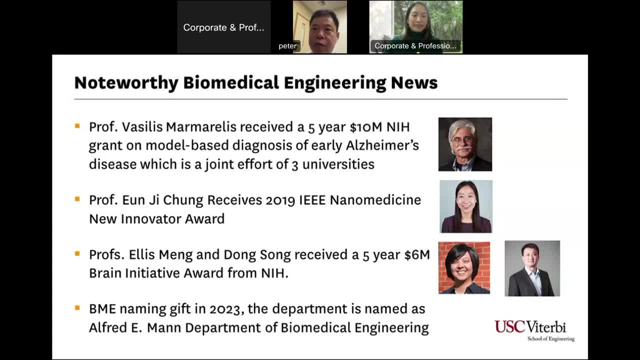 students, as well, as you know, to provide support for more student activities, such as like symposium attendance and even, you know, really support students to organize their own conferences and activities within the campus and, of course, reach out as well. next slide, please. so in terms of the 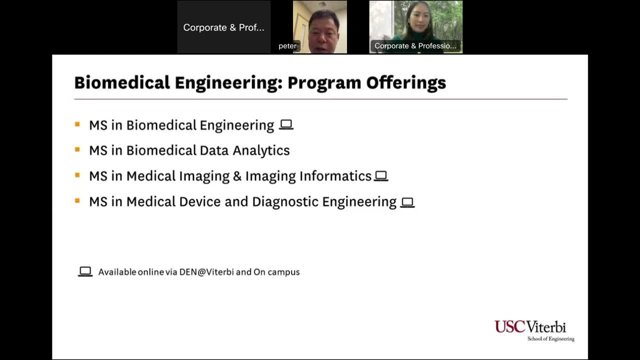 program of the biomedical engineering or the masters. we have four tracks at the current stage, but we are of course continuously revising this plan and there will be more coming up. so in general, currently we have biomedical engineering track, biomedical data analysis track, medical imaging, imaging informatics track and the device, medical device particularly- and diagnostic engineering. 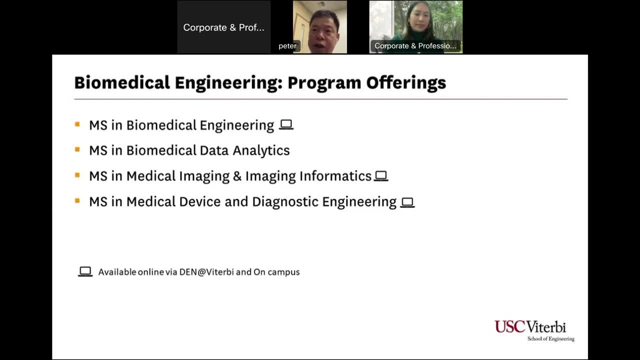 track. we are considering to add ai machine learning. you know track as well in the future. so if you're interested, you know by all means you can reach out to us. we are. you know we're working on that. hopefully it will become a reality, you know, later this year or next year. next slide, please. 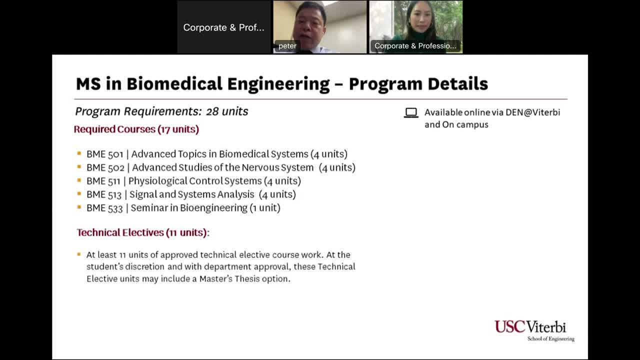 let's see. hopefully you can allow me to see more. so basically, you know this is the track about biomedical engineering. you can see we have 28 units and there's required courses, five courses, which is 70 units. 17 units essentially to cover, you know, the general topic in biomedical system. 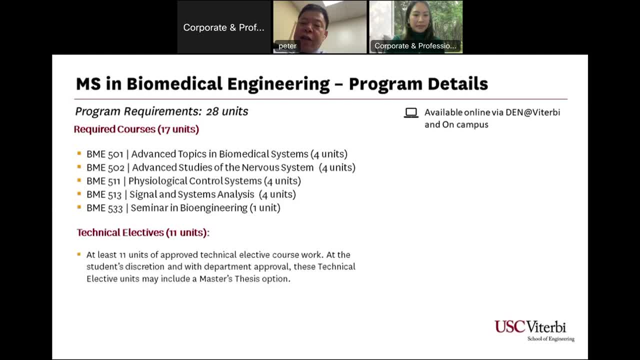 neural nervous system, physiological control system, signal and system analysis. and there's one seminar, you know, in bioengineering, which basically we invite different faculties, you know, across nation and frontiers, across the nation and you know even some of them are from the international. you know universities basically covering all the different topics you know, and we have a lot of different. 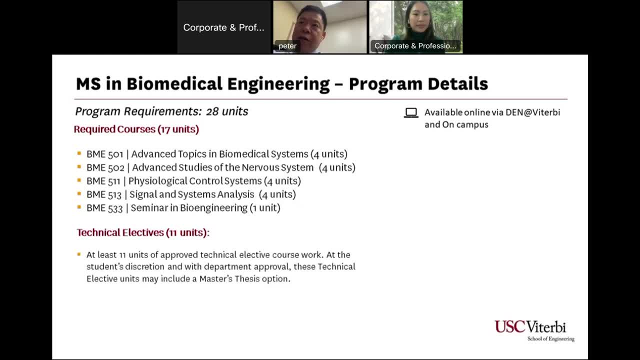 courses. so all those courses are in our department and they're in the department at the university of texas, and so we have three courses, which are the transition and the online courses, which is different from the other two, and then, after the course, you can also have the choice for. 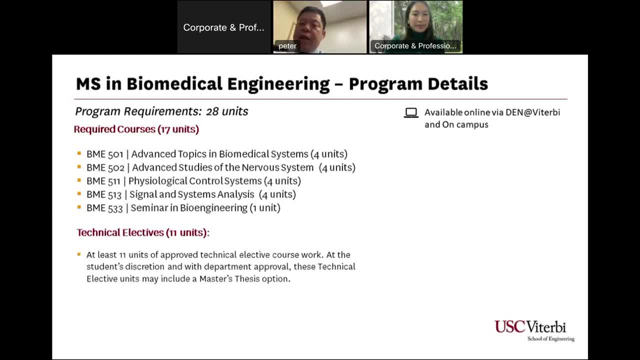 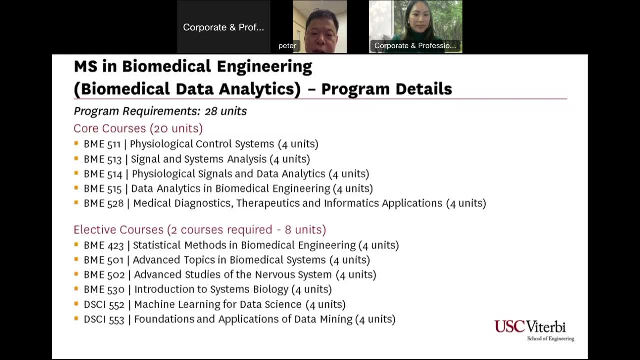 technical electives. that's basically you know you have multiple choices as long you can. you know certify having units. so that's the biomedical engineering track. and the second would be: you know data analytical. you know program, again, 28 units total and you take these. you know core courses, five courses. you know majority of them are. 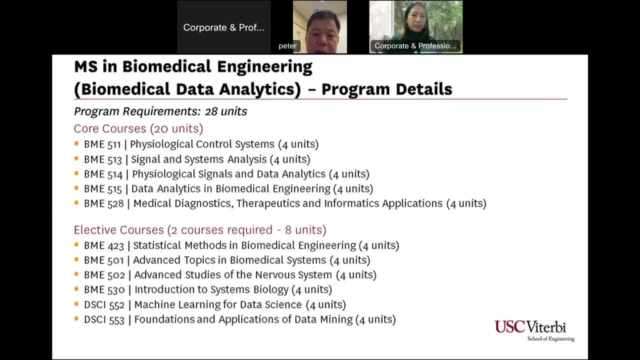 very similar to the overall design. and then you have the choice of electives, right. so for the electives you can really, you know, based on your own interest, you can pick, like, for example, two courses from all these you know elective courses, based on your own, you know, preference. 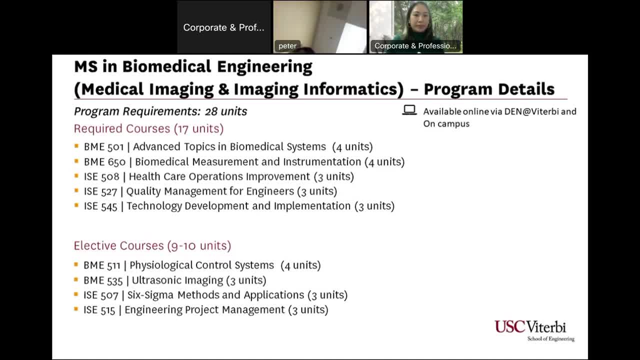 next piece, the medical imaging, imaging informatics, similar design. it's always: you have the base, you know core causes, right, 17 units and you can see that there's some common causes like these advanced topics in biomedical systems. but there will be some, you know, like, like. 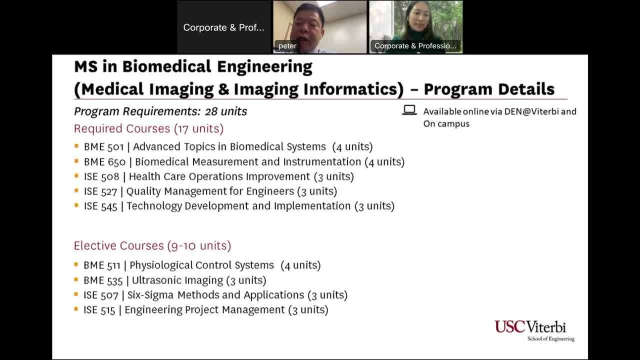 really unique courses like healthcare, operation improvement, quality, imagine, management for engineers and technology development and implementation. so these are the core which you are required to take and then after that, again you have the choice based on your personal preference. you can choose like from these different courses to satisfy these nine to ten. 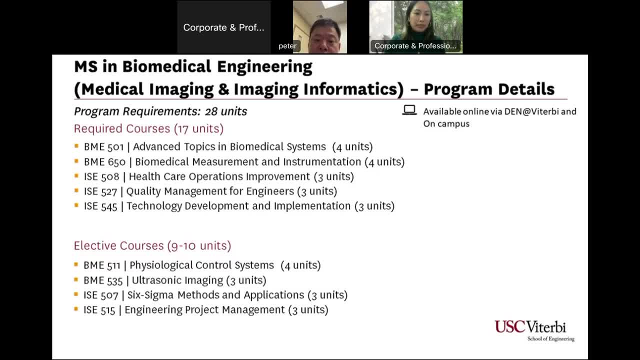 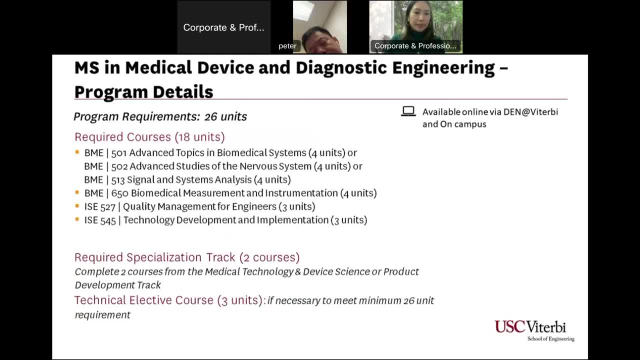 units. essentially it's like two or two and a half, you know, courses, uh, next piece. okay, so this is the other track which is, you know, focusing on the uh, the medical device and the diagnostic engineering. again, you know you have a core which is uh five plus actually six courses. but 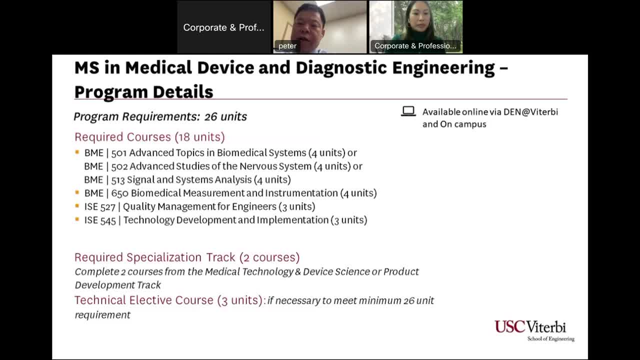 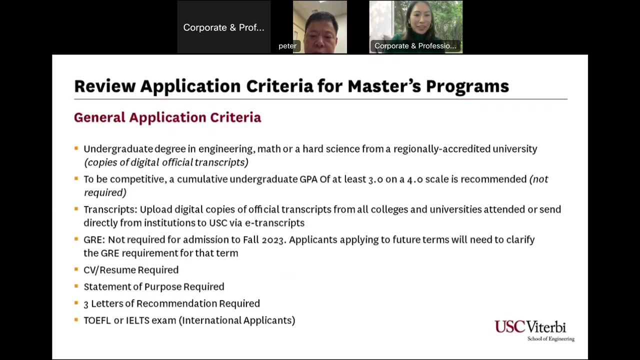 some of them are, you know, like three units uh, so you satisfy uh with this uh requirement and then take another like two courses. you know, basically, in the elective, you know options. again, this is your choice, depending on your interest. uh, next piece. thank you so much, professor wang. um, okay, yeah, i could go ahead and go through the um, the. 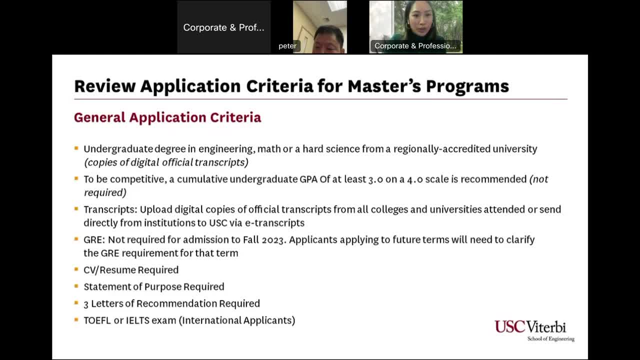 application um for the masters program, um. so yeah, thank you, professor wayne, for walking us through um. you know the different biomedical engineering programs and also um. you know kind of what the curriculum is. so for those of you you know who are interested in um, in applying um, the general 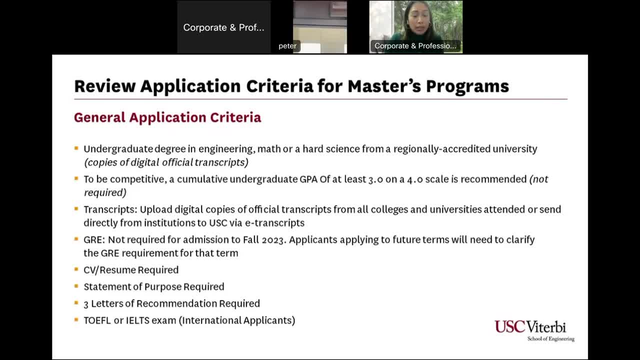 application criteria would be um for our programs. um would be a having an undergraduate degree in either engineering, math or hard science from a regionally accredited university. so for the application purposes, thank you so much for joining us today. we're going to move to the next slide, please. 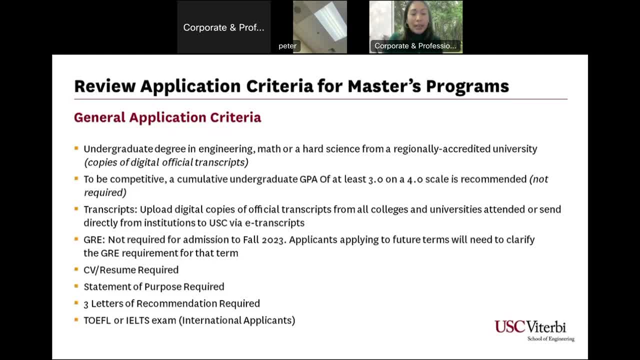 you do need to submit your digital official transcripts And, to be competitive, we do recommend having a 3.0 GPA on a 4.0 scale, but by no means is it a requirement. but it is highly recommended And, in terms of transcripts, as I mentioned, it has to be from all post-secondary. 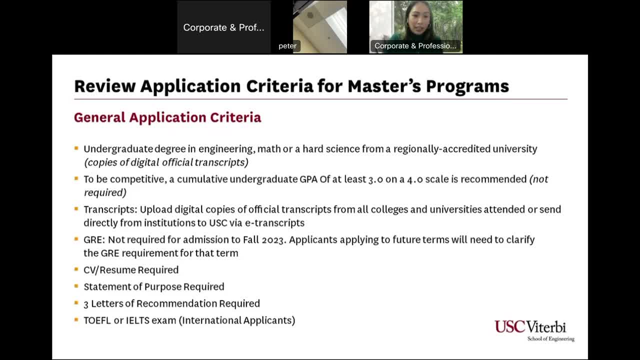 universities Anything after high school. you will need to submit digital copies of your official transcripts. Please do note that you know the GRE is not required for admissions to fall 2023, you know. but we do recommend you know if you are applying to future terms especially. 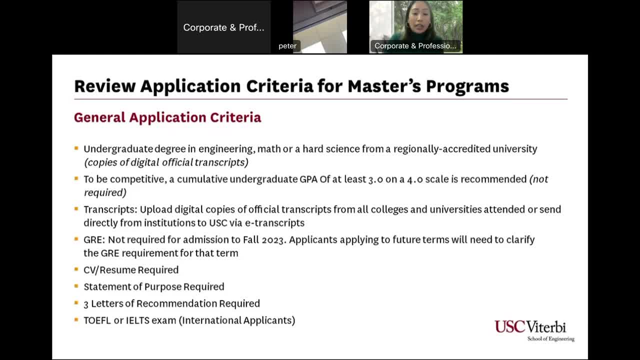 you know, if you are watching this webinar at a later time, to just clarify on our website whether or not the GRE would be a requirement, And then for all our graduate programs, actually, you know, it does require you to have a CV or a resume, and also a 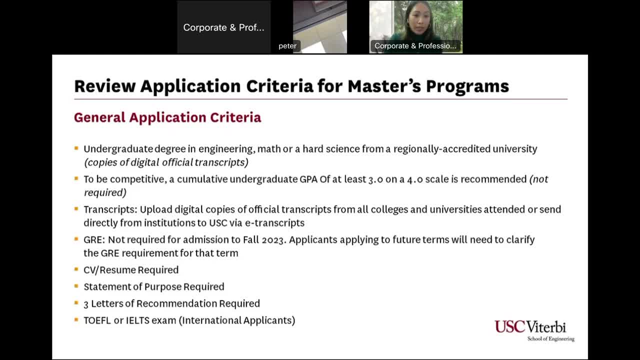 CV. So for students who are looking to apply for the GRE program, you do need to submit your statement of purpose, so like your personal statement, and then also three letters of recommendation are also required as well, And for those of you who are international applicants, 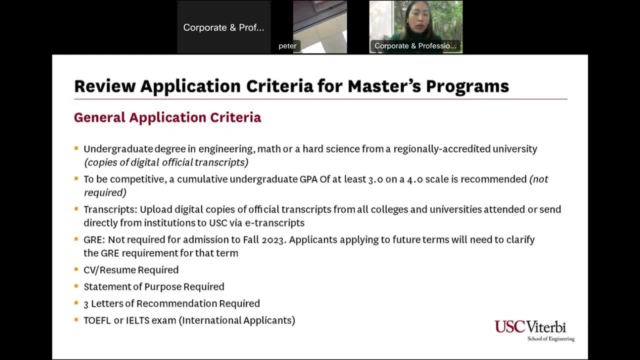 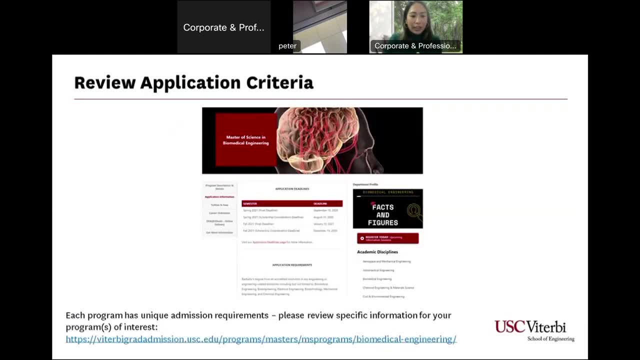 you know, there may be a chance that for international applicants, you do need to submit either your TOEFL or your IELTS exam. So if you, you know, are deciding that you want to, you know, So you know. we do encourage you to go to our website and to look under the individual file- medical engineering program page- for more information in terms of the admissions requirements. 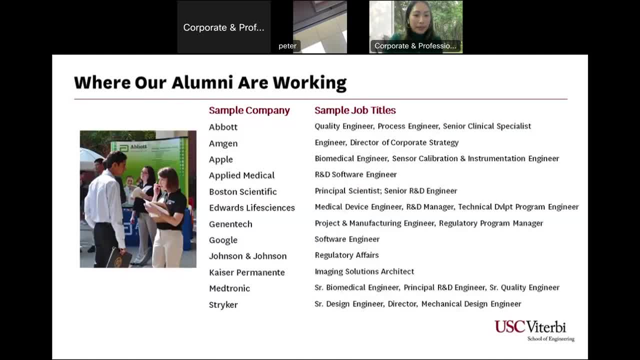 So, Professor Wayne, would you be able to to walk us through you know where some of our alumni's are working now, who have graduated from the biomedical engineering programs. Oh, you're, you're, Can you unmute yourself? Okay, perfect, Yeah, so all students goes to a different. uh, you know areas mainly, uh, I think it's about a half half. 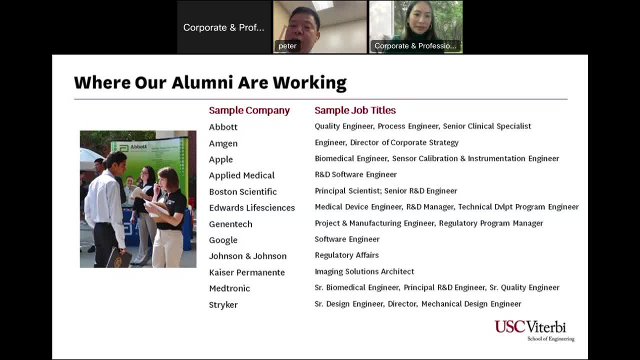 Uh, some of them, you know, continue to go to the graduate school And uh, a larger portion of them also will go to industry Right. So these are the listed uh like, uh, you know uh, outcomes. 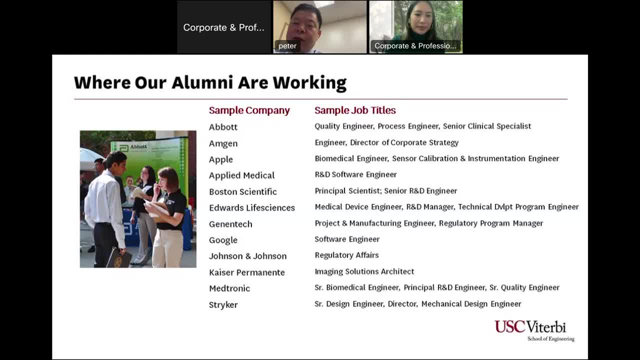 Our student go to the about emerging April. you know I don't want to. you know, read the other names, but you can see these are mostly a pharmaceutical industry. you know, by technology in some of the medical companies essentially. 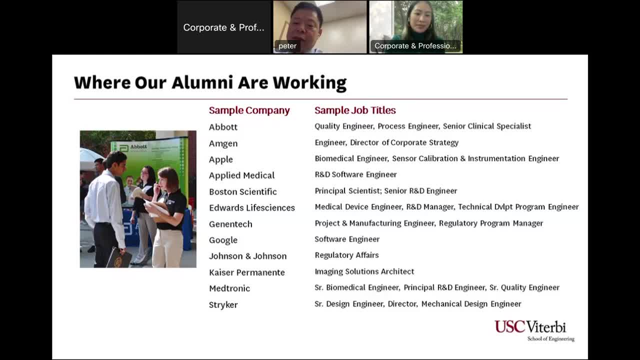 And they serve as engineers, uh, you know, in these different companies. Uh, and the student. The other portion goes to graduate school, like the, become a master's student and also somewhat, I think one-third, perhaps- directly getting to the PhD program. so these are the most outcomes for the. 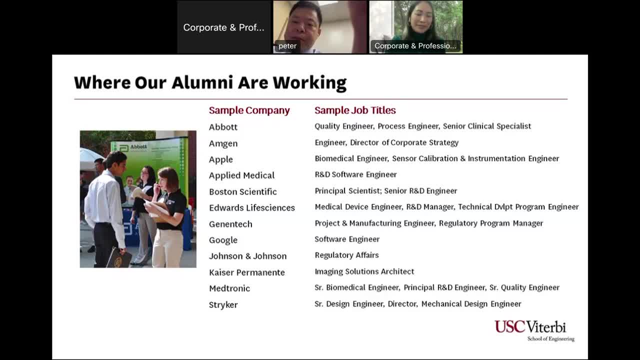 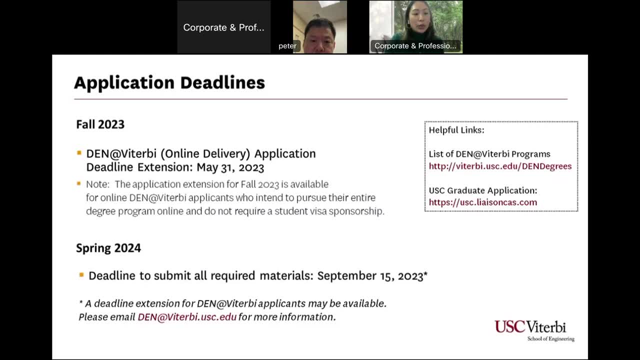 student from the department. thank you, professor way. so, in terms of, you know, application deadlines for those of you who are interested in applying for fall 2023, which does begin, you know, mid, mid to end of August, we have actually extended the application deadline for online den of a trippy students to May. 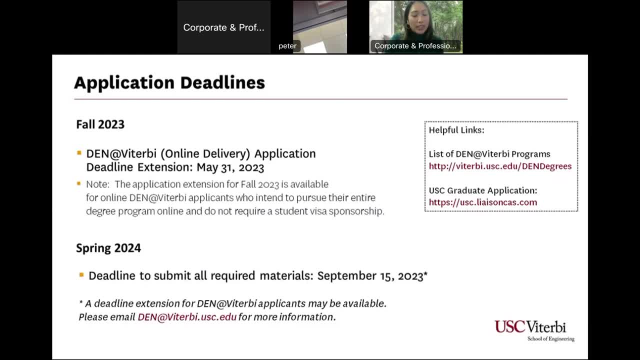 31st, and so, to be eligible for this application extension, you know you do need to be pursuing your program online as your delivery method and also you know you can. it's also for students who do not require a student visa sponsorship, such as a f1 or i-20. but you know, for those of you who are like you, 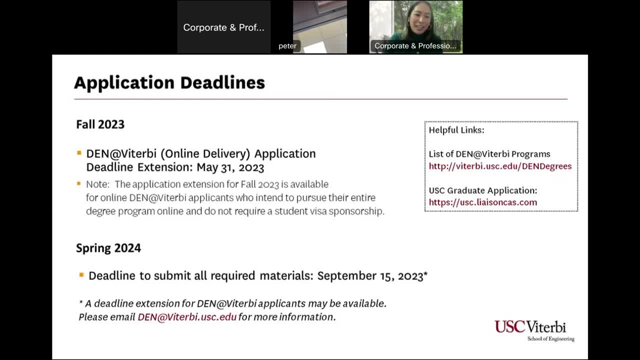 know, fall is just too. it's too soon. I need a bit more time. our next semester is coming up and we're going to be doing a little bit more of that. so if you know, if you are interested to pursue as an online den of a trippy student, we do. 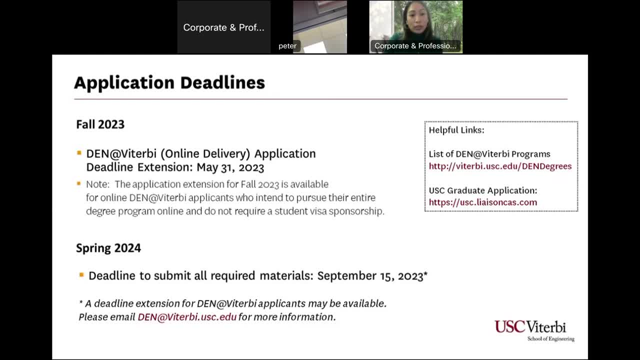 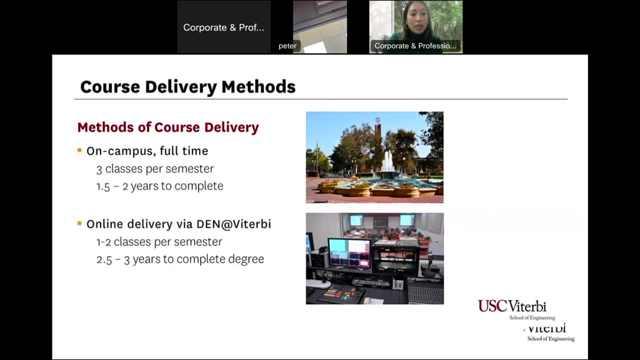 have a application extension available. so please do reach out to me at that email identity- uscedu- and I'll be able to work with you on that. so, in terms of the course delivery methods, so you know we do have two different course delivery methods. so we do have two different delivery methods. so we do have two. 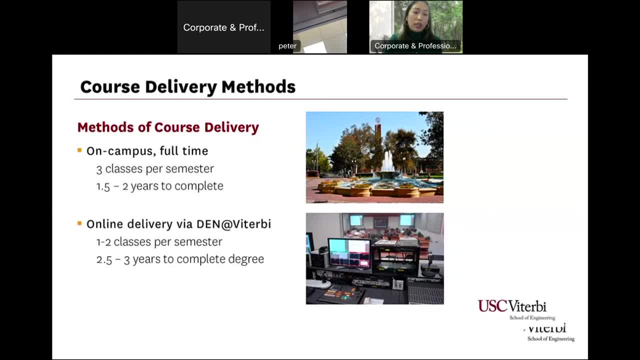 different course delivery methods. so we do have the on-campus and then also the online through den of a trippy. so on campus, you know just really quickly it does the students who tend to pursue on campus, they do tend to be pursuing it at a full-time basis, which means that you know they aren't working and they're. 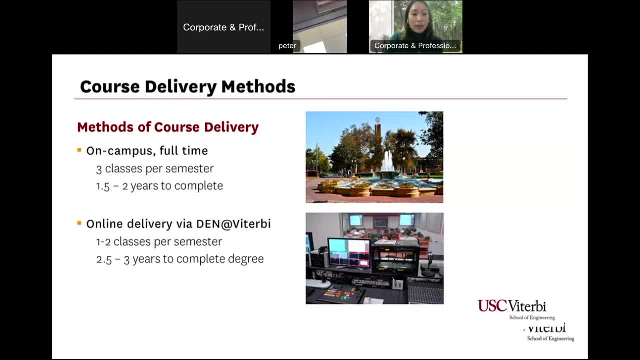 taking around three to four classes per semester, so then it would take them around maybe one and a half to two years to complete their degree, whereas, you know, for online den of a trippy students, they do tend to be working professionals. you know who are working on a full-time basis, and so they do tend 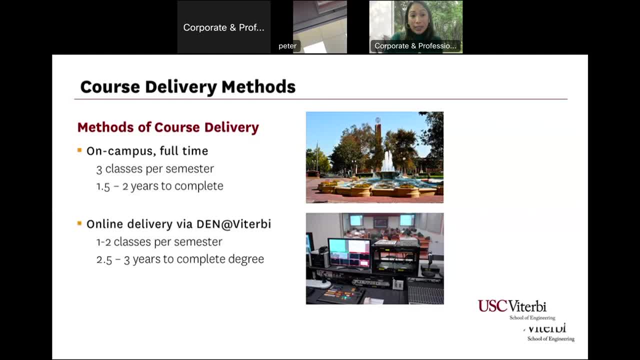 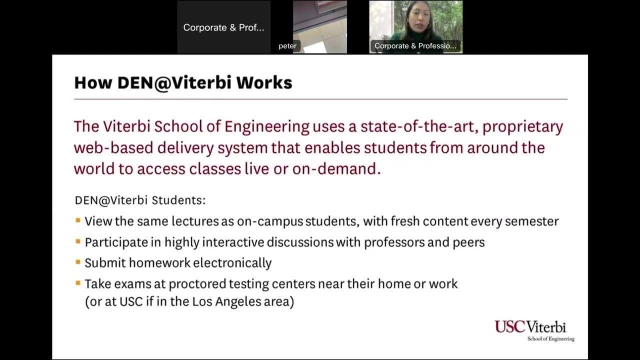 to pursue their graduate degree, you know more, on a part-time basis, and then they take one to two courses per semester, in which resulting in around a two and a half to three years to complete their degree. so how does den of a trippy work? so, for those of you, you know, who haven't joined us before, for a den of a trippy, 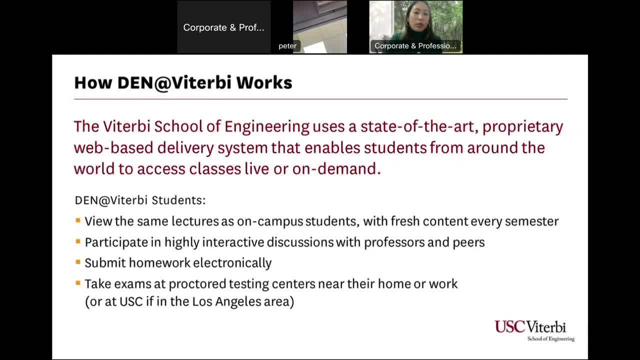 information session. den of a trippy is a trippy school of engineering. den of a trippy is a trippy school of engineering. you know own state-of-the-art, proprietary web-based delivery system which enables our students from all over the world to be able to access classes in two ways. 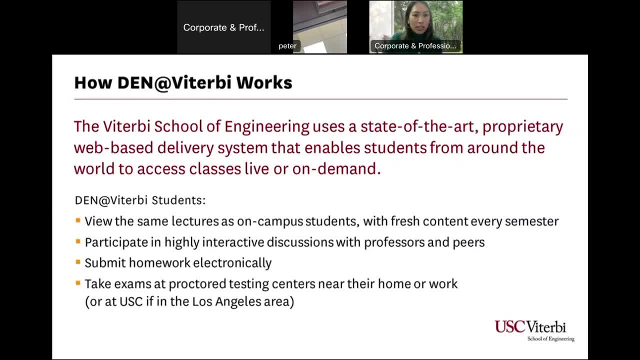 One as it is happening, so they are able to stream. stream it live, watch it live as it is happening. They can interact, raise their hand, they could dial in or they can watch it later as a recording on their own time, as because it is really flexible, especially for working. 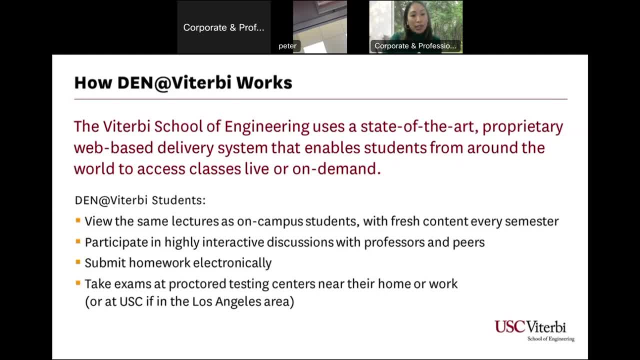 professionals And also if you are a Denver Tribute student, you know you can also sit in on classes as well at USC's Los Angeles campus if you are ever in the area. So that is also another flexibility also. So as a Denver Tribute student, so you do view the same lectures as on-campus students. 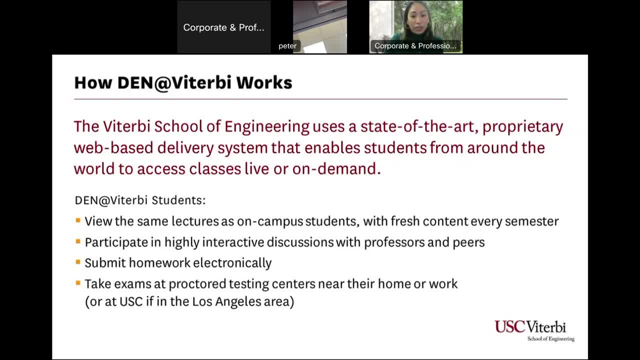 So you know the curriculum is the same. It is also fresh content every semester, So what that means is that the faculty will bring in content that is trending during the current time. So then industry professionals, for example. you know they are able to apply what they. 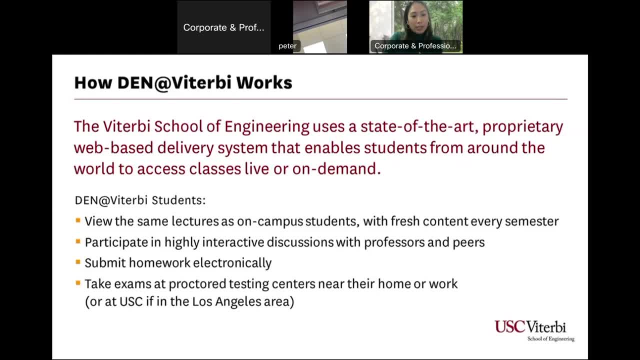 learn in the classroom to their day-to-day job. And then you do also participate in highly interactive discussions with your professors and your peers and you do submit your homework electronically. And then, in terms of exams, so exams, you will be taking them at a proctor testing center. 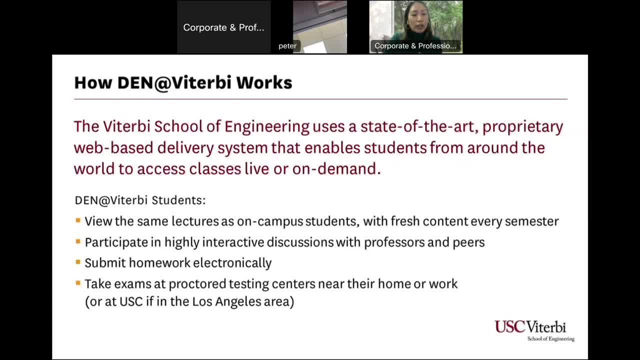 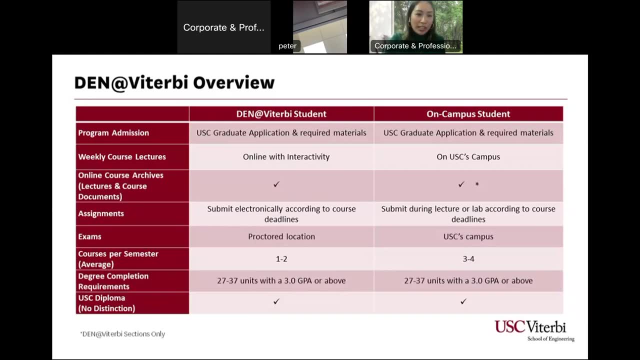 located near your home or your work. But if you are living or residing in Los Angeles area, then you would actually take your exams in person at USC's campus. So for those of you who are joining us live, or watching this as a recording afterwards, 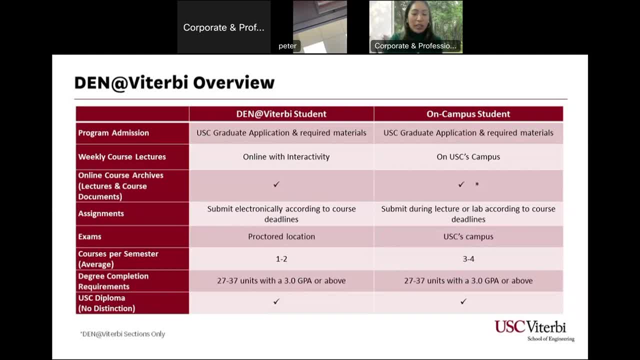 and you are, you know, unsure whether you want to be a Denver Tribute student or an on-campus student. you know, this slide here is really to show you that you can do that. So if you are a Denver Tribute student or an on-campus student, you know this slide here. 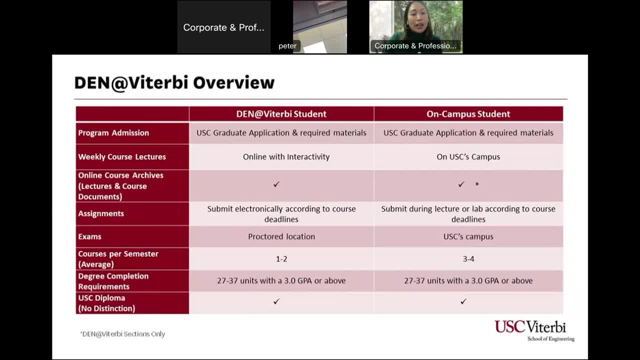 really is to show you what the difference is. As you can see, the program admission requirements are the same for both delivery methods. it is more so in terms of the course. lectures are different. As you can see, online students do have online with interactivity, but as an on-campus student, 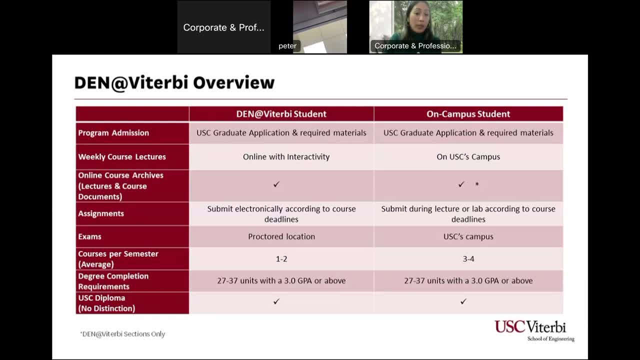 you will be expected to be sitting in lectures in-person. And then, in terms of having access to online course archives, as an online Denver Tribute student, you do have access to an opportunity to take an on-campus class at a off-campus, But as an on campus student, you would only be access to um to course archives only if you are enrolled in a den of a trippy section, which means that there is a den student in your class. in terms of assignments, 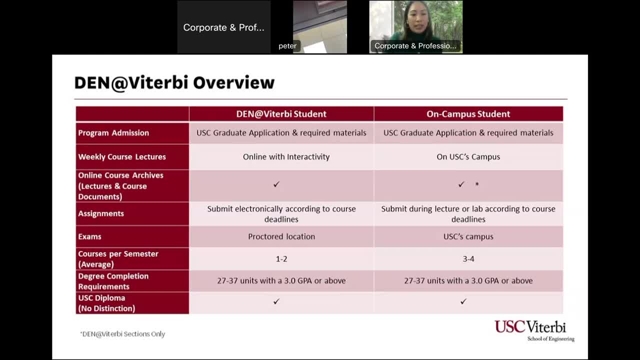 You know it is electronic for all my students but then for on campus student you will be submitting it in person during the lecture or lab. But do note that the course deadline dates would be the same. exams for den of a trippy. 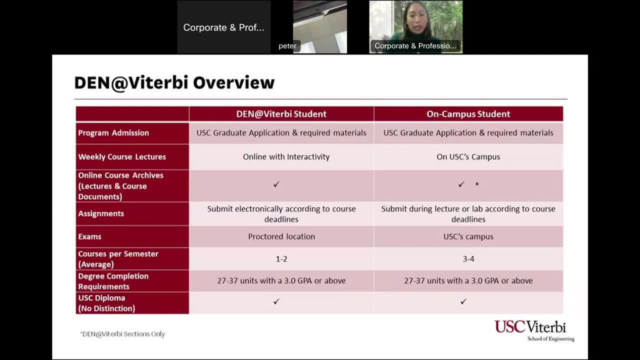 Student it would be at a proctored location, whereas on campus student will be taking it at Los Angeles at the Los Angeles campus courses per semester I talked briefly on before online den of a trippy students. you know they do tend to be working professionals, So they do tend to take 1 to 2 courses per semester And then the degree completion requirements are the same for both. 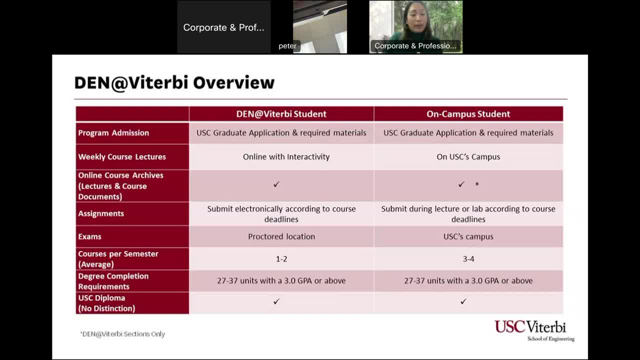 You do need to achieve a complete degree, completion requirements Um a certain amount of units, and you do need to have a 3.0 GPA or above. So ultimately, at the end, the degree that you um and diploma that you will receive from USC, it will be the same. 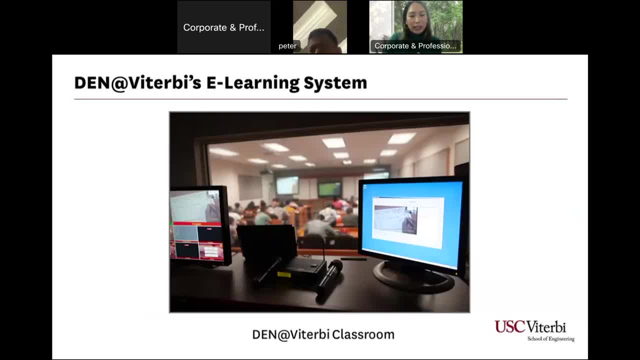 And this is just really quickly. you know a um how our den of a trippy classroom books for those of you who are interested in pursuing your degree as an online den of a trippy student, And there's just some additional information- So limited. 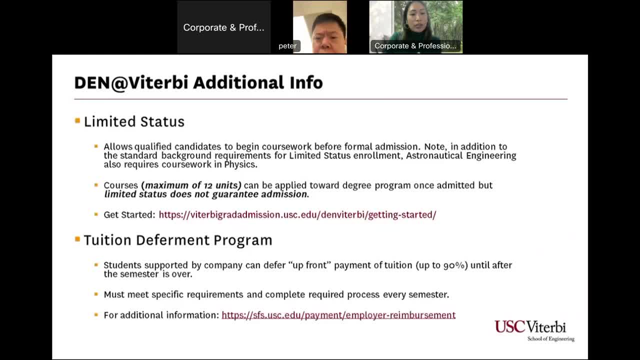 So we do offer a limited a status enrollment option, and so this is a enrollment option, you know, which really allows our qualified candidates to begin their coursework before formal admissions. So you do need to have a 3.0 GPA to be able to to enroll and jumpstart as a limited status student to take some courses. 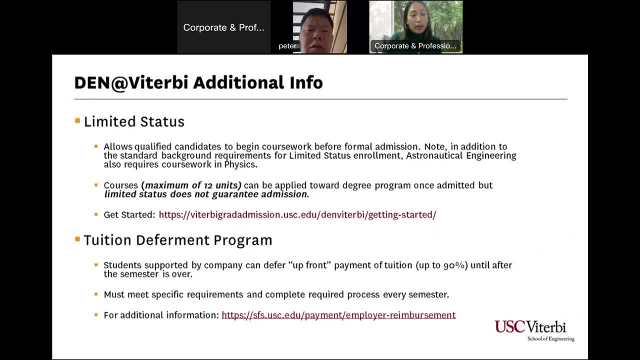 And for those of you who are being sponsored and reimbursed by your employers, we do also have a tuition deferment program, which means that you are able to Defer your payment- your upfront payment of up to 90%, until the end of the semester is over. 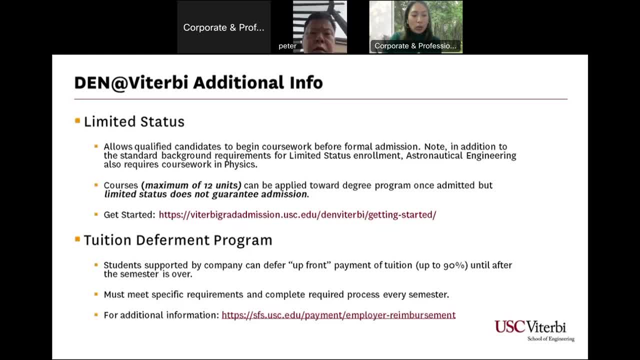 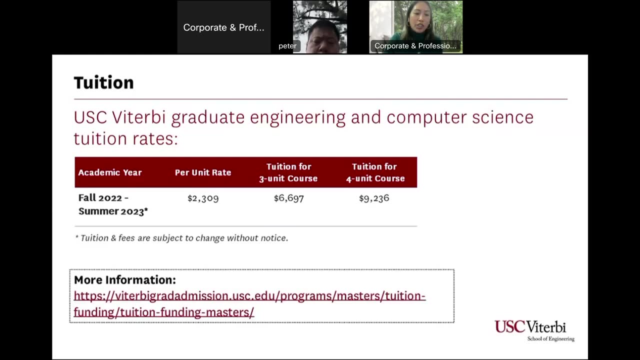 So for any more of this information of limited status or tuition, tuition deferment program, I do recommend you to visit those links that we have indicated on this website. I just really quickly, just to cover on the tuition. So the tuition at USC Viterbi for graduate engineering programs. 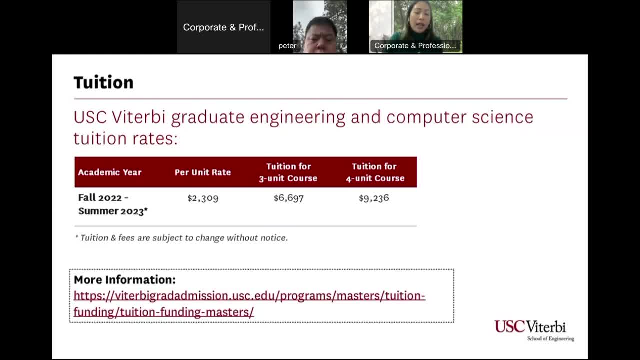 is uh 5 per unit rate, as you can see here, and so this is the current rate as of today. do note that the tuition rates do change every academic year, So we do recommend for you to go and go to our tuition and funding page on our website to reference the latest and most updated tuition fees. 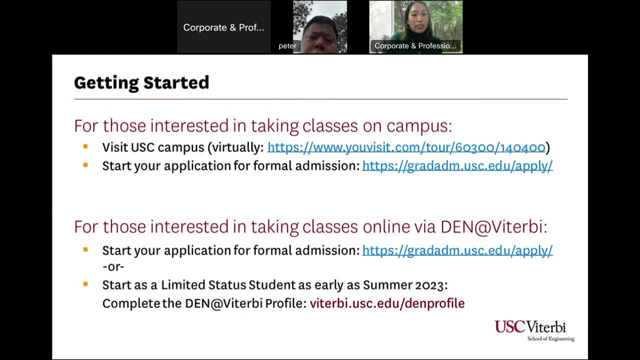 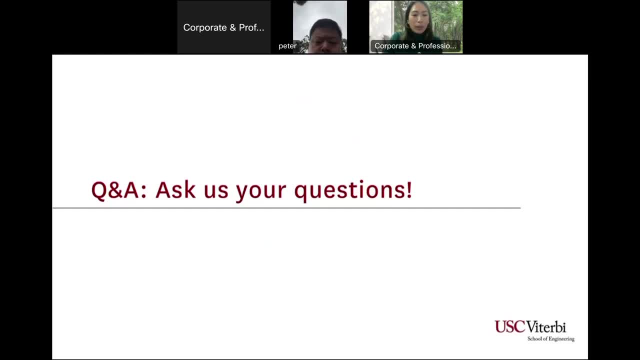 And so for those of you who are looking to get started, you know, here are just some helpful, Some helpful links for you to navigate. Okay, perfect. So let's go ahead now and, you know, ask some questions to Professor Wang. 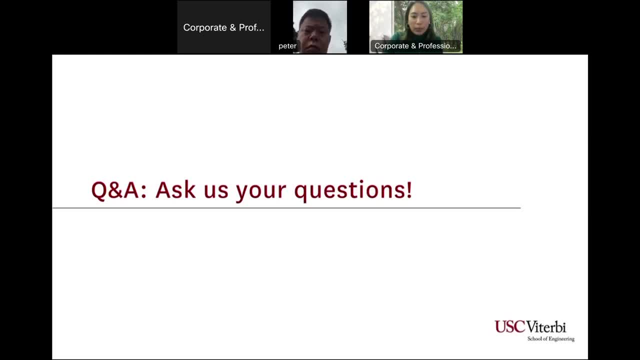 So, you know, meanwhile we'll let some people start typing in their questions. but you know, Professor Wang, I do have, you know, a question for you. you know, Are there any opportunities to do any research or thesis? 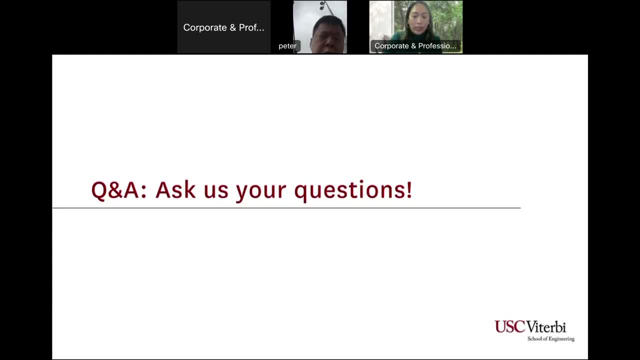 Um, you know, related for people who are interested in biomedical engineering programs as either as a on campus or online student. Uh for sure, Okay. So even in my own lab you couldn't have three masters students doing research in my lab, and I'm sure there are many others. 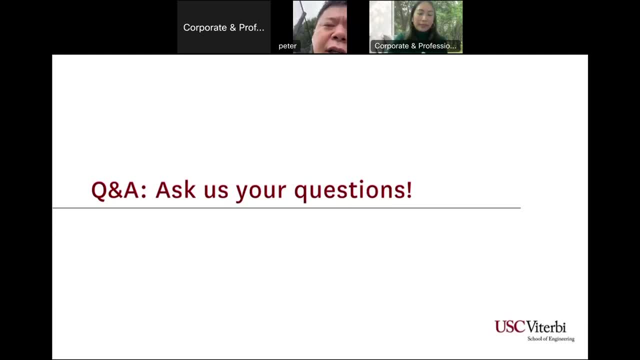 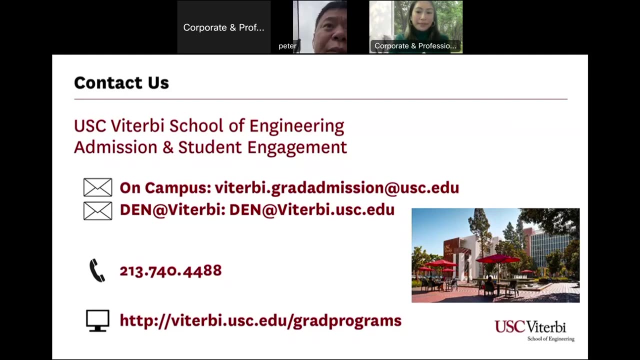 you know in other faculties and colleagues in the department And because we have a large full or the courtesy faculty, so it's very easy for students to find out. you know the laboratory and have some research experience. for online students that may. 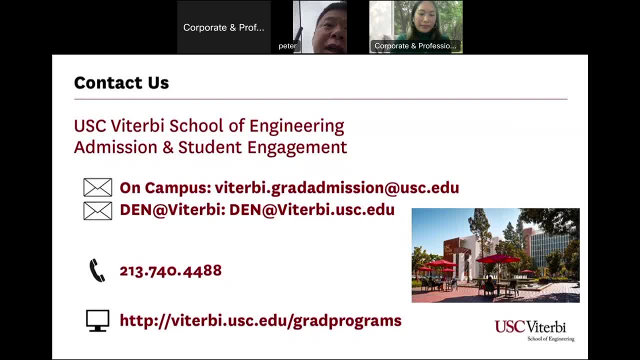 you know, create some kind of you know limitation because they can only work on research related to, like informatics and database analysis, those kinds of things that you know. if you want to have real hands on experience, then it probably would be difficult. 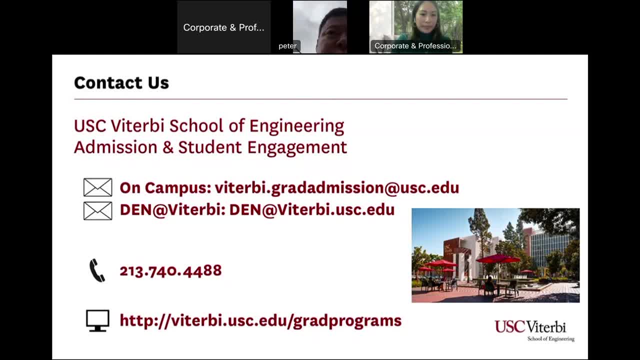 but we do have some like working on, like more you know, modeling and analysis. Perfect, Thank you. Find out more information? Okay, perfect, Thank you so much. And so another question would be, you know, so another question would be: 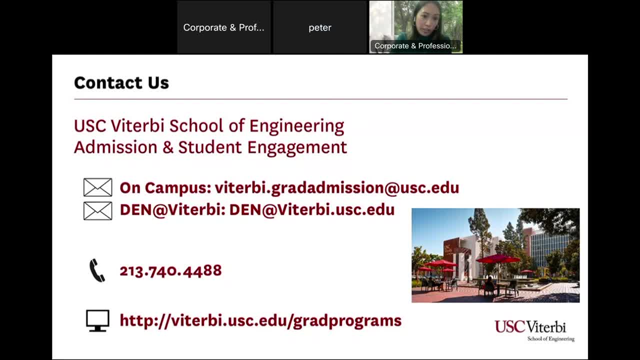 you know, if someone was was able to complete their master's degree in biomedical engineering and they want to pursue a PhD afterwards, you know, is that, is that possible? Of course it's possible, So for actually it's a. 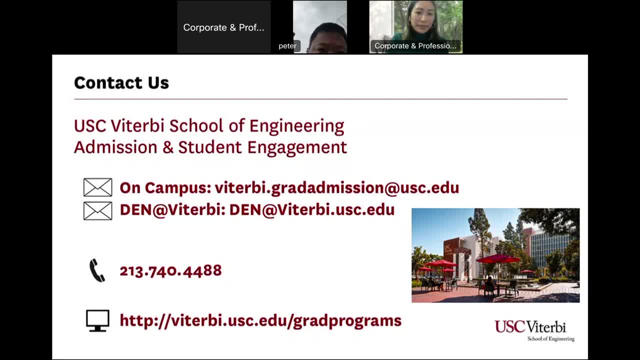 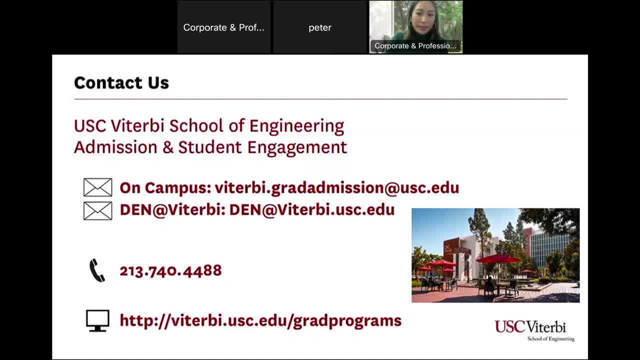 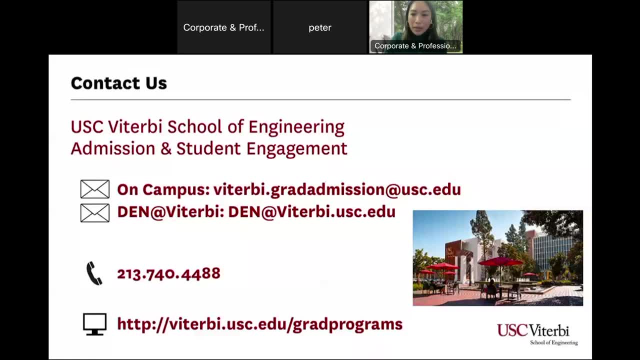 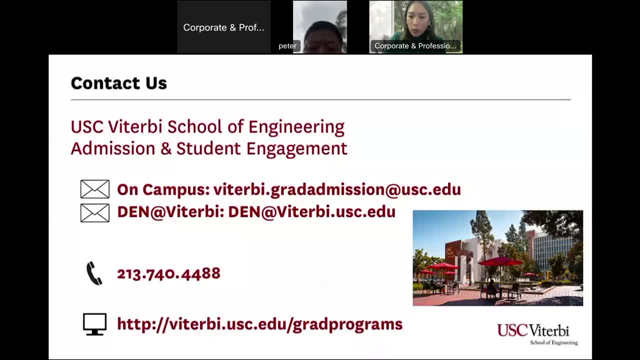 that came in from one of our attendees. Um so, what is the general consensus for future applicants who want to sit in on lecture before beginning? Um so, um, I think this is actually more for us here in the admissions team. Okay. 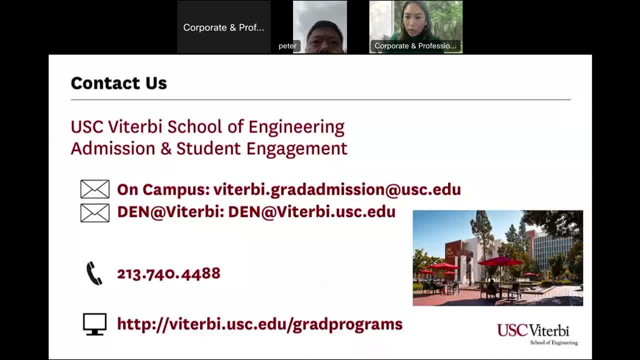 Um, okay, So, Karina, so actually, yes, So, um, if you're interested in, you know, sitting in on a lecture before applying for formal admissions. unfortunately, you know, um, that wouldn't be. we do have. 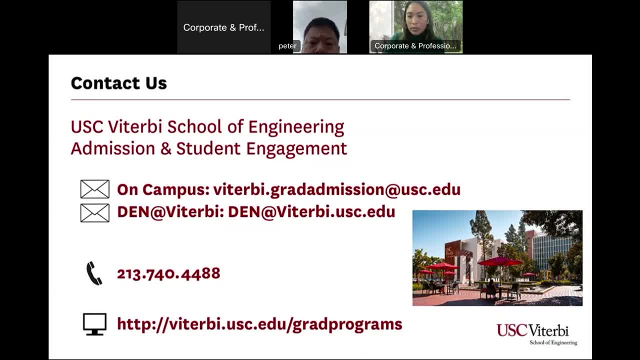 you know some options that are available, but then you would still need to um. so one was, for example I mentioned would be the limited limited status. So limited status, you know you can take 1 course, for example. 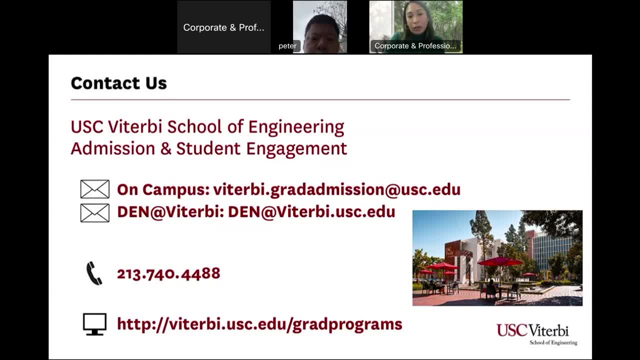 in biomedical engineering to kind of feel out, you know, whether you're interested in that program by taking a course. So it's, it's a way for you to kind of jumpstart before applying for formal admissions. But you would still pay the tuition fee for that 1 course that you would take for that semester. 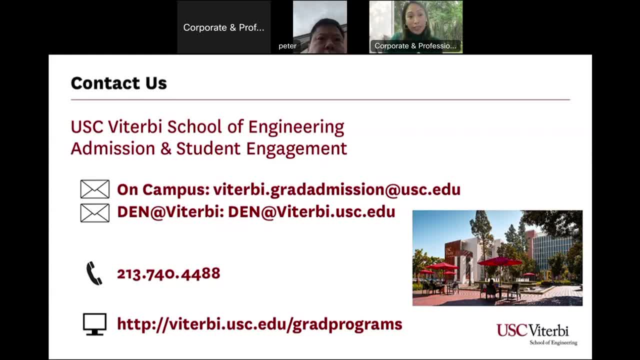 Um, so with limited status, you can take up to 12 units as limited status before then apply for formal admission. But you know, even if you, if you take 1 course during 1 semester and you decide that you want to enroll for more emissions, 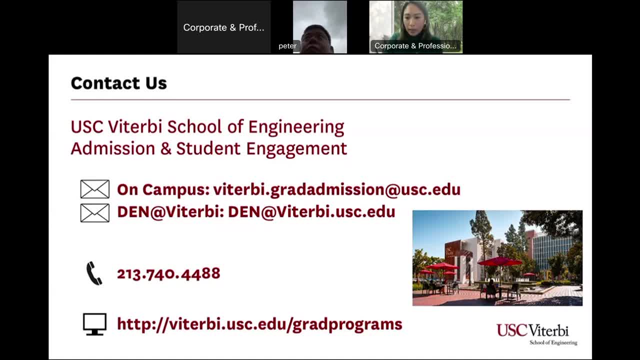 then you can definitely do so And um, okay, so if the application process, yeah, so the application process is the same for in person students, so for on campus and online delivery method, you still need to complete the graduation, The graduation application form, so that it is the same, and but just note that for limited status, that is, that is, for online data to be to be an online delivery, 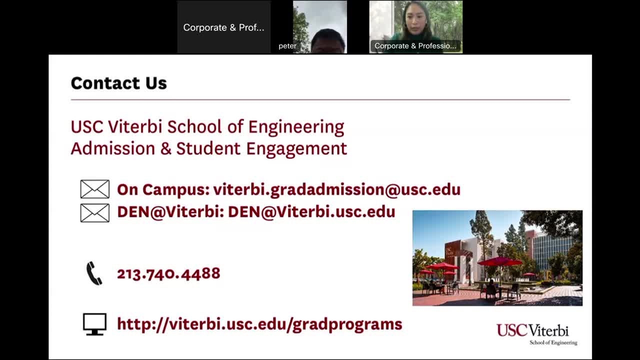 So limited status is for online delivery method only. Okay, So you work at full, you put you, you work at tech, but your schedule is somewhat flexible. Is it possible to do online in person classes? Yes, most definitely So, as I mentioned, you know, as an online data. 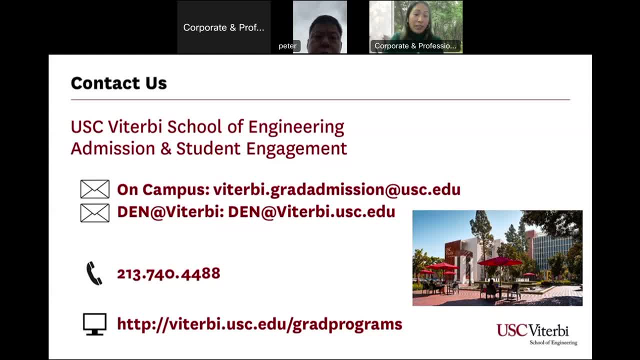 a student, you do have a physical seat in every class that you are enrolled in. So you know, given that you are based, you know, at tech, you know which is probably in the downtown office or like campus- you know you are able to fit in on classes. 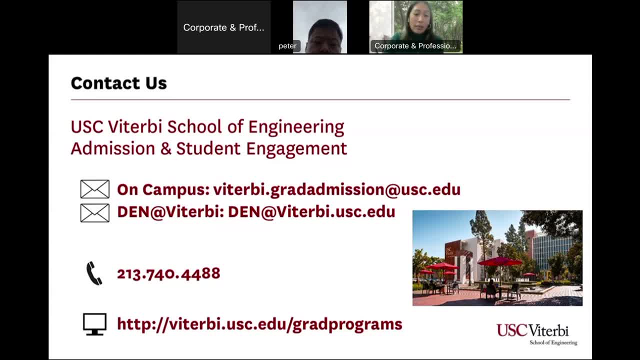 If, if you have the flexibility and your time allows- but you know, by no means is it a requirement, but it's definitely that benefit. Um, Okay, so I do, Okay. So, Professor, when we do have a question. so, um, this is a question about hands on experience. 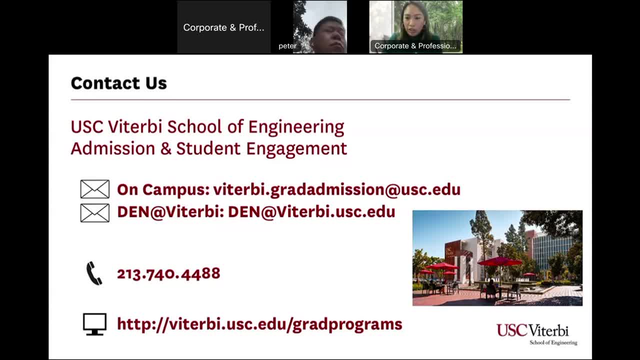 Are we partnered with other colleges or what or where do you recommend getting hands on experience? Yes, uh, can you hear me? Yes, yes, we can hear you. Okay, Yeah, we can hear you. for hands on experience: Yes, 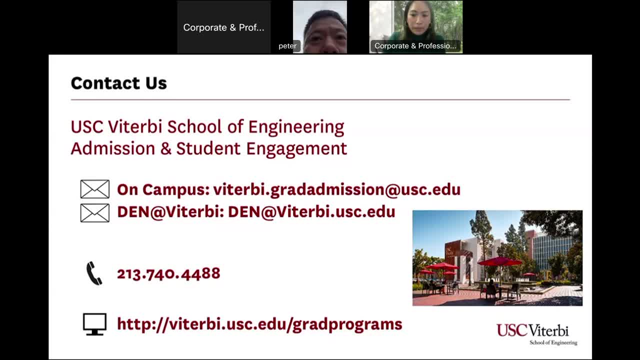 Uh, the most common way is: uh, you reach out to, uh, you know, you change your radio faculty or and start to do some research and immediately You have access. there are some classes. they have some portion of the hands on experience. 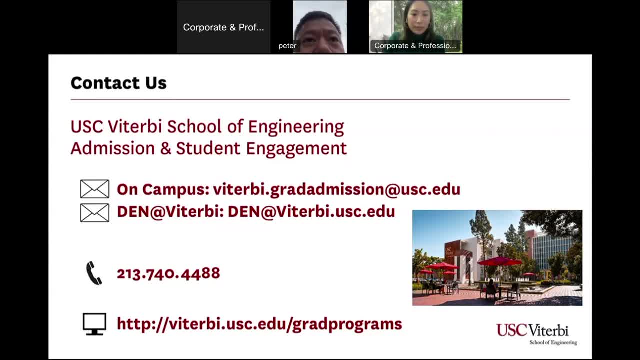 In fact, I'm going to also create a class. you know, uh, perhaps there's a 1, 3rd or even more you know classes. we will basically focus on some projects which student will be required to operate, some like portion or the experiments. 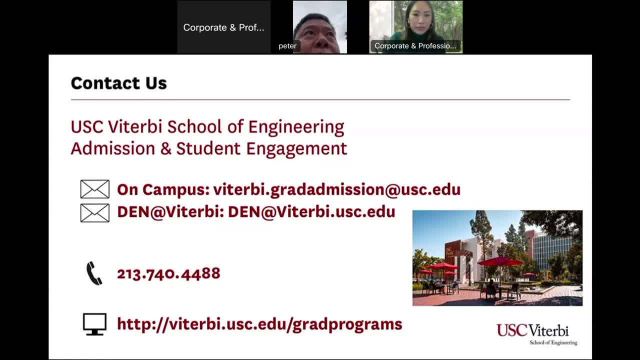 So those are all possibilities but mostly, I think, most convenient or easy way just to reach out to different factors and do some research in the laboratory. that's most substantial and we have so many faculty for you to, You know, explore. Thank you for that, Professor Wayne. So there's a follow up question from um, from the same attendee who asked the question about hands on experience. So, um, they are currently residing in Houston, Texas. 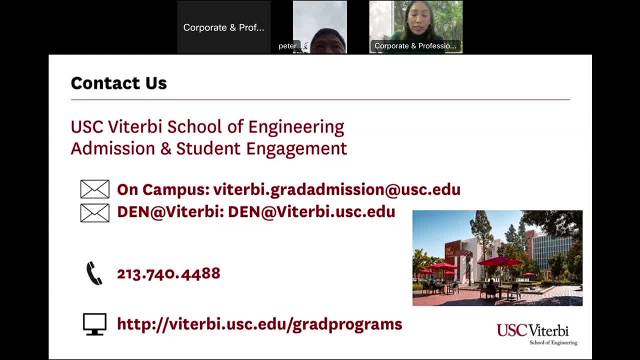 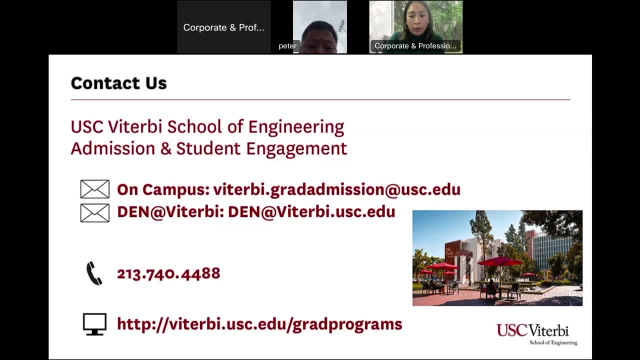 um through USC, through the program, or if we're partnered with campuses nearby. Professor Wayne, we can't hear you. Hello, Hello, um. well, I can see Tamika um, in general, for We'll wait for the way to come back, but you know, just in general, for online data to be students, you know if there are courses where it requires you know hands on experience, or even like lab work, for example, where you need to be in person. 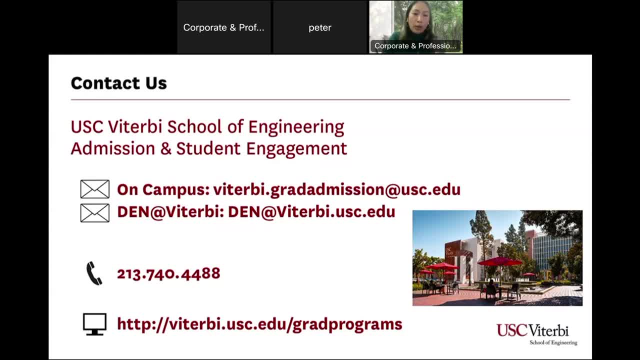 It. if it is a required course, then there will be an alternative for you to take. But unfortunately, you know, if it is a lab work, for example, which may be a elective, you know there are times where it won't be accessible on online. 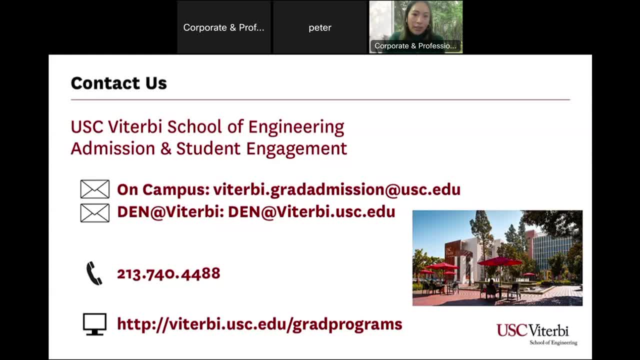 Through, just given the nature of the lab work and the course itself. So I hope that answer your questions. Okay, And in terms of can you hear me now? Can you hear me now? Yes, I can hear you now. Yeah, I can hear you now. 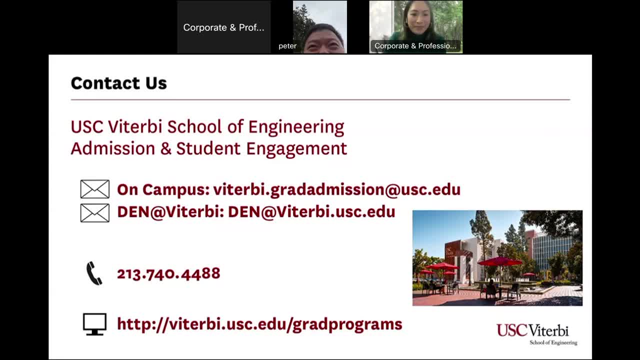 Yeah, Sorry, I don't know why, Maybe the question is so difficult- Internet, But anyway, well, would you like to? would you like to add on to that? Yeah, I think that's a difficult- you know, online to have hands on experience. 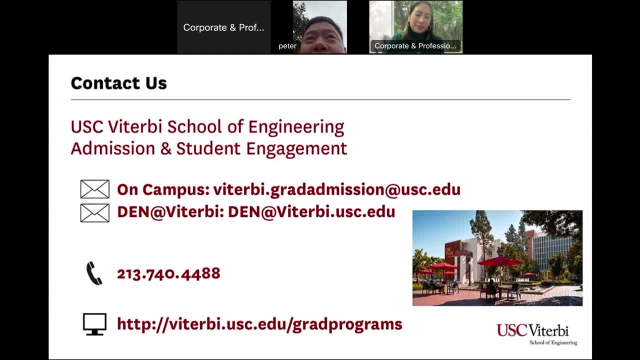 Uh, I think you know. again, you can talk to individual PI. They may. They may come up with some creative ways, but in general it's not that easy. Yeah, that's a reality. Sorry about that, Yeah. 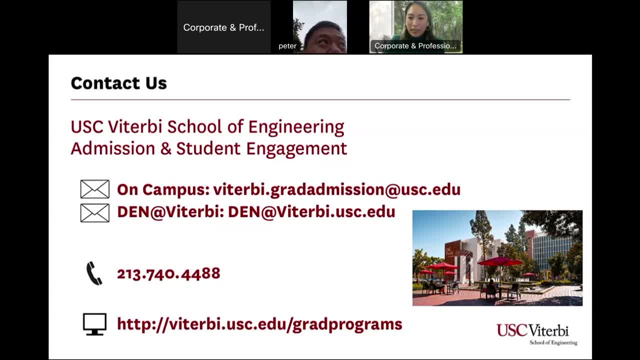 Yeah, Thank you. Thank you for adding on to that and confirming that as well, Professor way, Um, okay, So, um, there's another question which I could, yeah, which I could answer. Um, yeah, So, whatever you want to sit in in lectures to get better acquainted with the material, just in general. 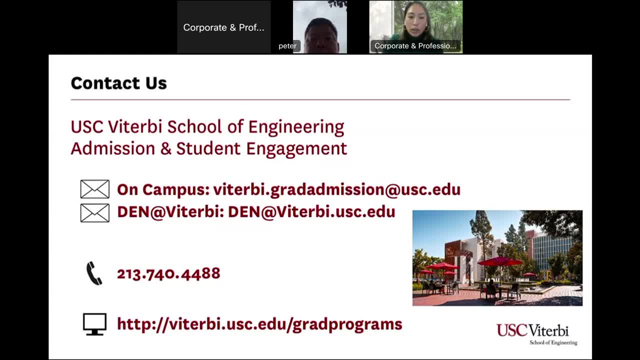 Yeah, So, um, so we Do offer, you know, a, we do offer a audit enrollment and not it's not really enrollment, but it's auditing, Right. So a student who wishes to you know view a course for a non credit. So it would be non credit. 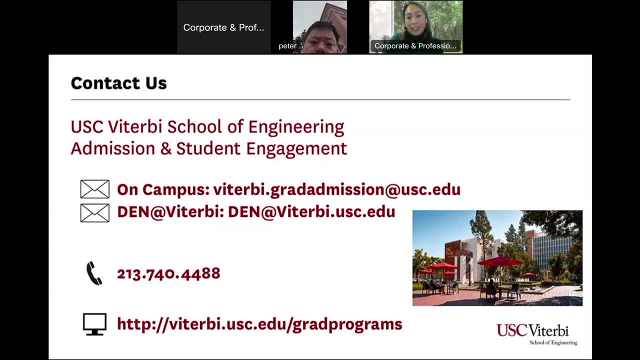 As a student and you know you can enroll as a audit student, so all the students will receive class materials. but then you do not complete homework and you do not take exams, So of course you know it's taken for audit. 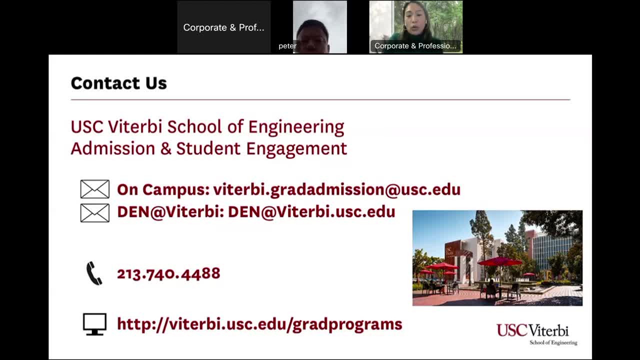 The course size taken for audit. you actually won't receive university credit and it also won't appear on a USC transcript or grade report, but you would still be paying the current tuition rate For that audit course. so I mean, I hope that. 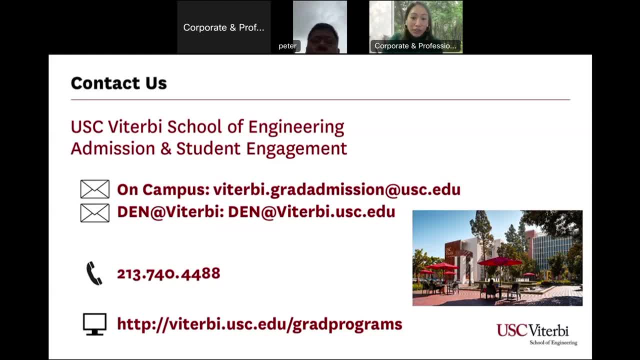 Also, you know, answers your question of the different options. So you know we don't have a Option where you just come in and sit in on a lecture for 1 time. There's basically Either you are a audit where you will come and audit the 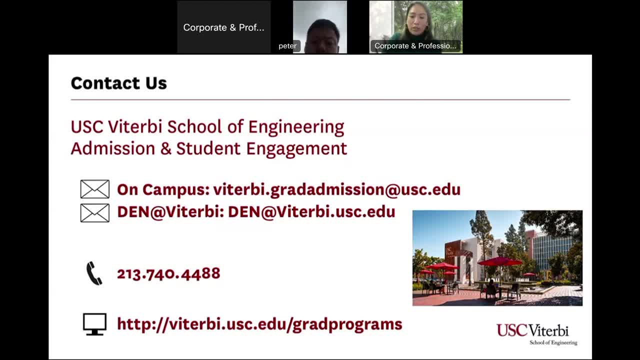 The course, but then you still need to pay a fee, as well of the current tuition fees for that specific course that you are auditing, or you can apply as a limited status, student or formal admissions. So I hope that answered your question. But you know, given that you know, our time is, you know, close to coming up. 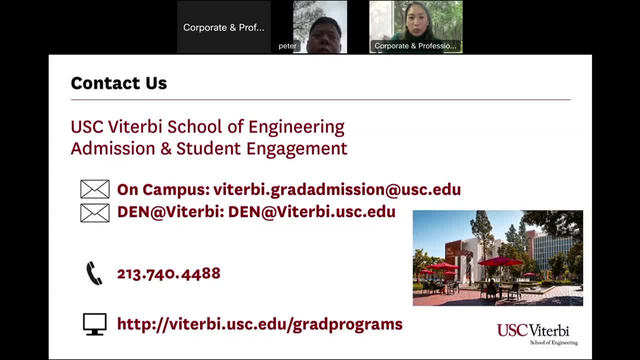 And you know. I just want to thank you know, Professor Wayne, so much for your time and just being able to to answer, answer our questions and to take us through this very informative webinar of the biomedical engineering programs. So, for those of you who have questions, please feel free to reach out to us. If you're interested in the on campus delivery method, you could reach out to our on campus team. If you're interested in online, you know you could contact me at